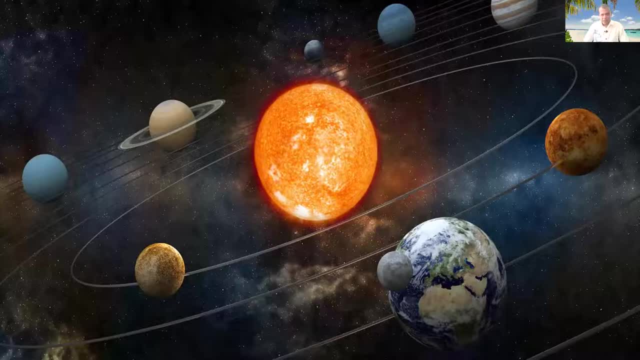 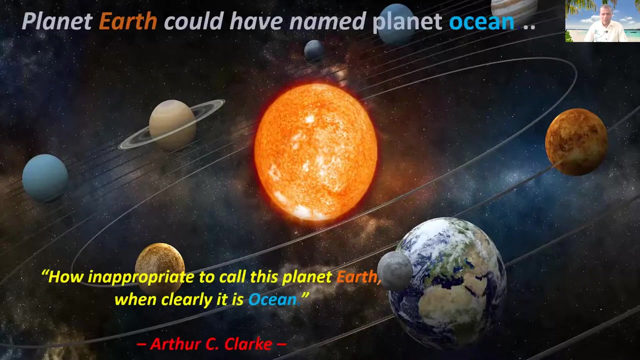 and you can see the Earth here, as with all the other planets. So Earth is not an unusual planet, It's just like other planets. But there is one difference in Earth. So what's the difference? Right, As once Arthur C Clarke said, we have given a wrong name for. 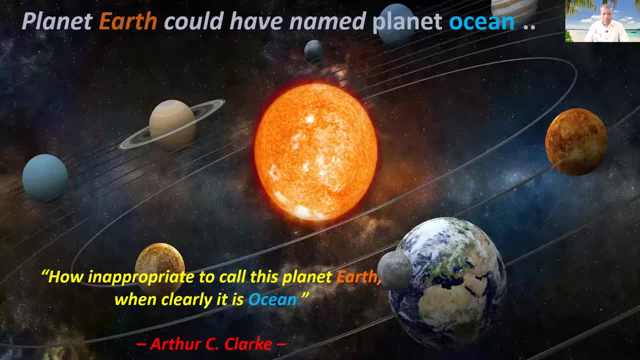 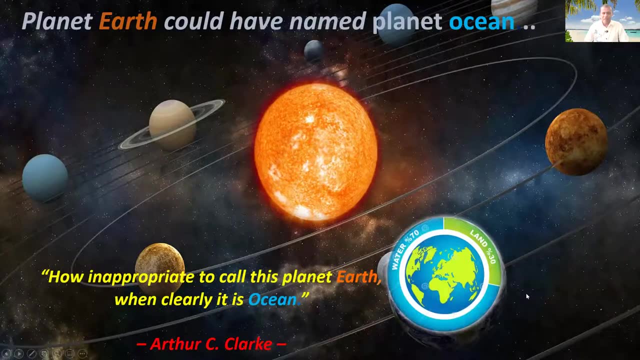 the Earth. How inappropriate to call this planet Earth when it's really the ocean. because why it is? the reason is that you see that 70% of the ocean is covered. sorry, the Earth is covered with both and just 30% of the land right, And if someone see from the outside, 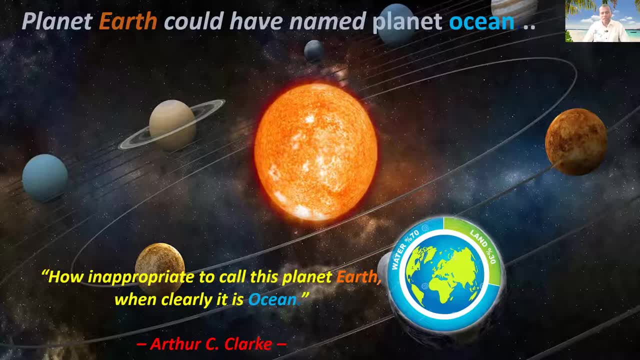 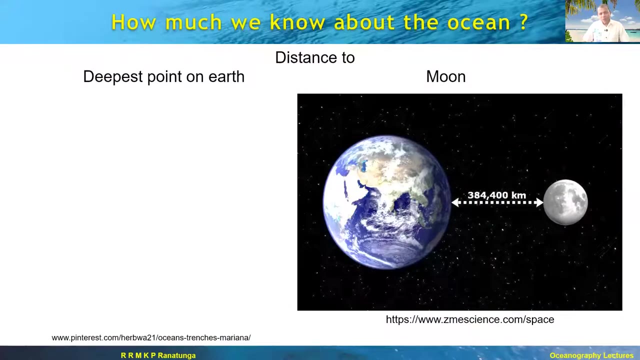 the Earth just look like a watery planet. It's full of water, Right. so this could have been called the ocean planet, But unfortunately we are given a wrong name right Now. how much do we know about the earth? Just to get an idea about that. 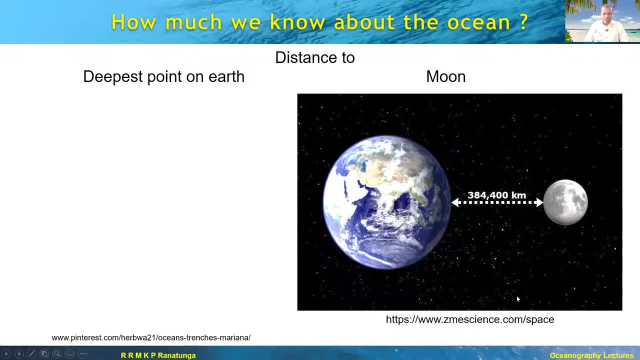 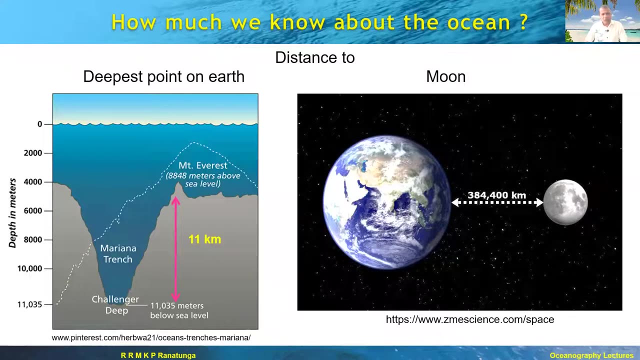 you can see this: the distance between the earth and the moon. right You can see how many kilometers there from earth to moon, And on your left you can see the deepest point, the known deepest point on our earth, that is, the Mariana Trench. 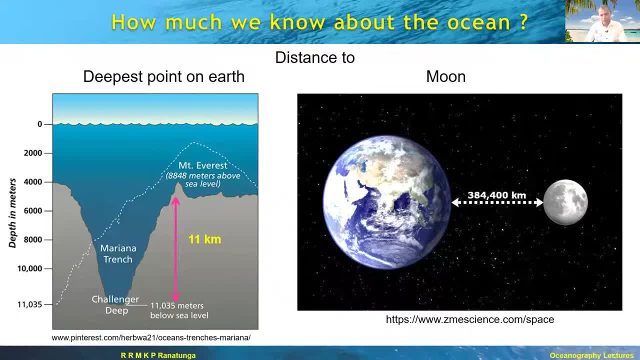 actually the Challenger Deep is the location in the Mariana Trench we call the Challenger Deep, So that is just 11 kilometers down. 11 kilometers. But how much we know about the moon and how much we know about the Challenger Deep? 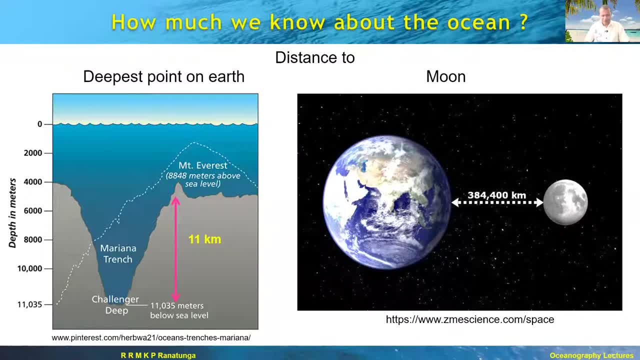 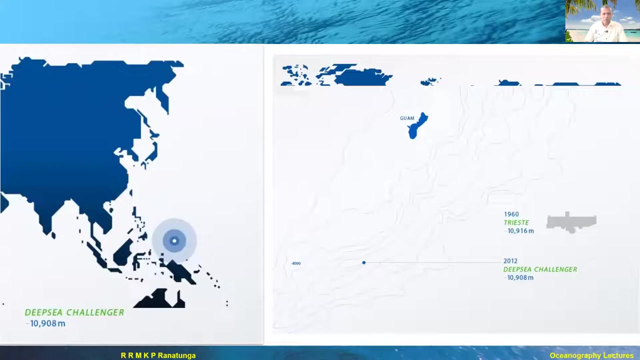 that is something to we need to discuss here. right, We know much better on moon than actually the Challenger Deep. that is our own earth. That is where the people paid very little attention to the like to learn about the ocean, So this is one of the issues. 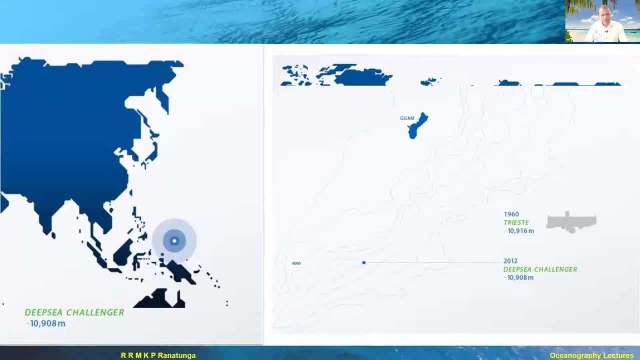 And you can see in this. this is the location where the Challenger Deep it is in the Pacific Ocean. as you can see here, the Australian New Zealand and the top. This is the area where the deepest point on earth right. 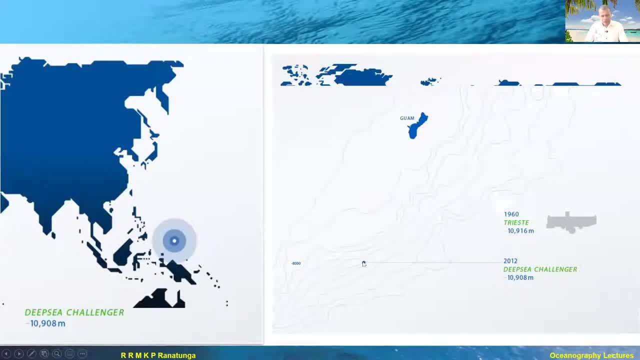 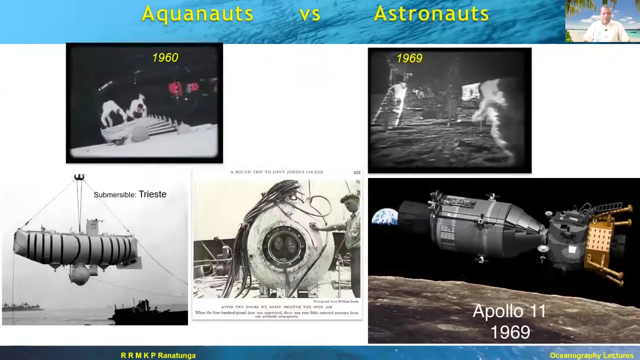 As you can see, here it is almost 11,000 meters, which means 11 kilometers down right. Right here I'm giving you an an comparison: the two set of people, or rather explorers, one group called the astronauts, right. 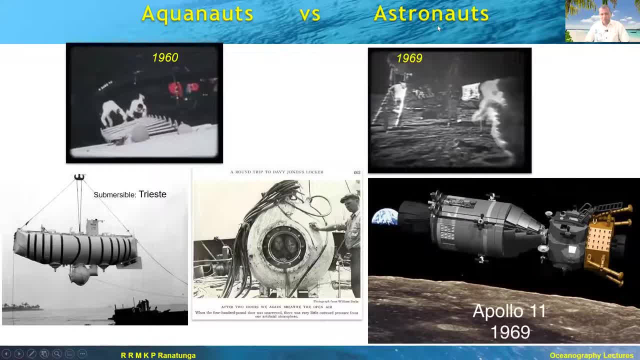 You've heard about this, the term- astronauts who are dealing with the, the, the outer space. but there are another group of people we less known. they are called equinox. probably you have not even heard about equinox, right, this term may be very new for you. 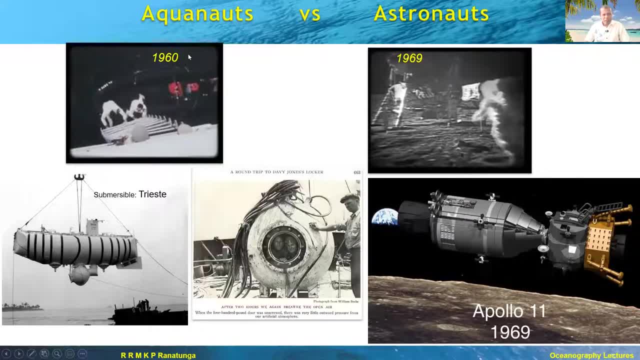 but actually the equinox started the expeditions, especially in the the deepest point on earth, that is, the challenger deep. that was in 1960s, right as well before you and even me. i was born right. they started this exploration in the challenger deep with this unique boat and an 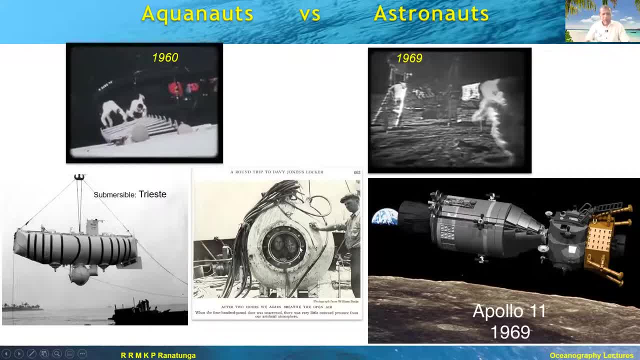 attached. something like this is a like a huge iron bowl where two people put inside- actually two naval people put inside that. actually it's a iron spear or globe providing the oxygen from the boat- right, you can see the boat here- and then for them to breathe, the oxygen has to come from the boat, because there is no. 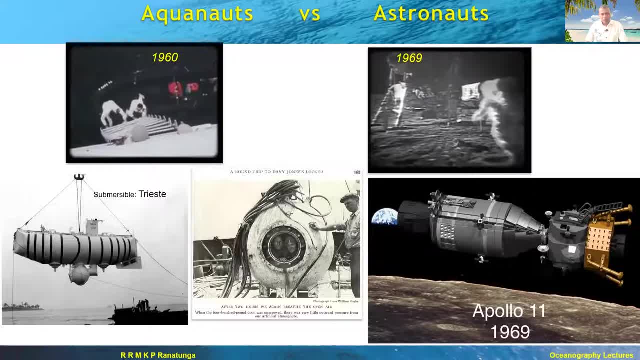 oxygen production inside. so with these two people inside in, with the small window for them to see, so they gradually lowered these two people into the deepest point on earth. that was in 1960.. so luckily they had no trouble. i mean, there's huge pressure inside but 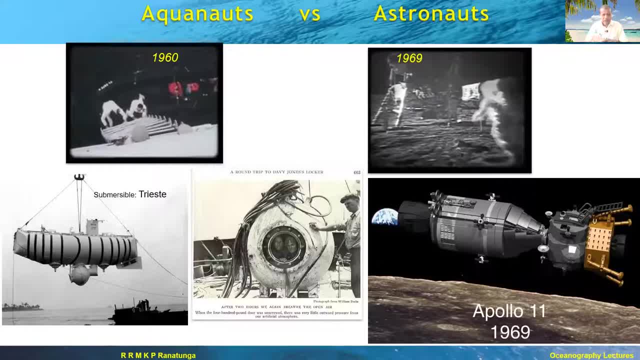 there were some cracks even in the the glass where they were looking at, but luckily there was no problem. they could come to the uh, to the boat again safely, right. so that was 1960 then for a long term after actually the people start going to the moon, that was. 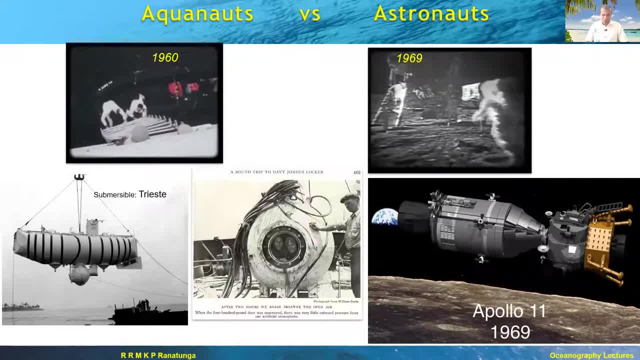 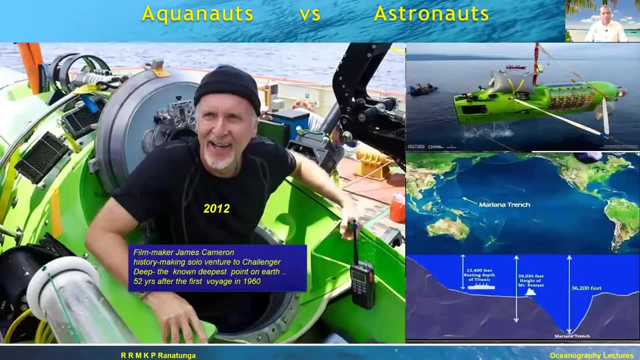 after nine years. that was in apollo. you might have heard about this on the expo apollo expedition. that was in 1969, after nine years of this initial exploration in the ocean right. but how long does did it take for a second person to treat it? 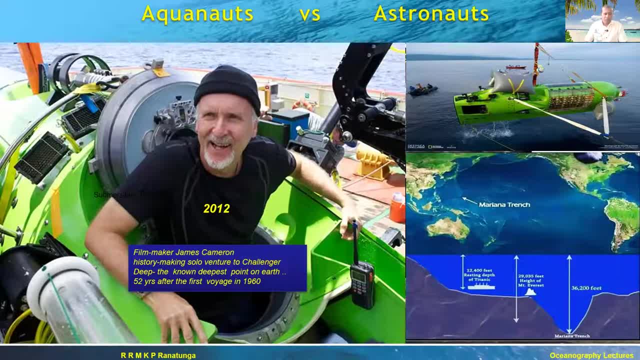 So you think you know, like, like you hadn't studied, if you didn't experience the dread and the gloom of theuelity yet, then they gained this important knowledge person to go to the the deepest point earth. right, we know, we have been several times to the moon. 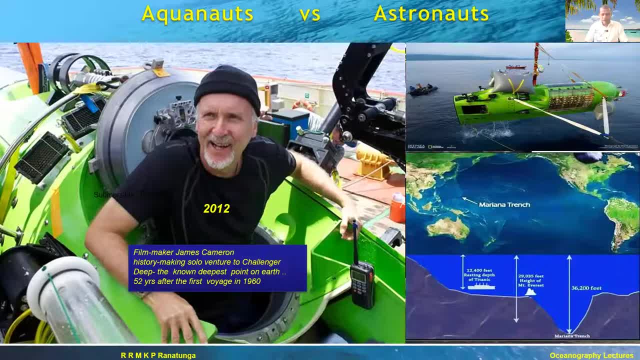 in between, but you know, first, the first expedition in 1960, right. the second expedition on 2012, right, it took more than 60 years. for a second right, uh, the expedition, that second expedition, actually by a well-known person. uh, you might have heard about this name: james cameron. 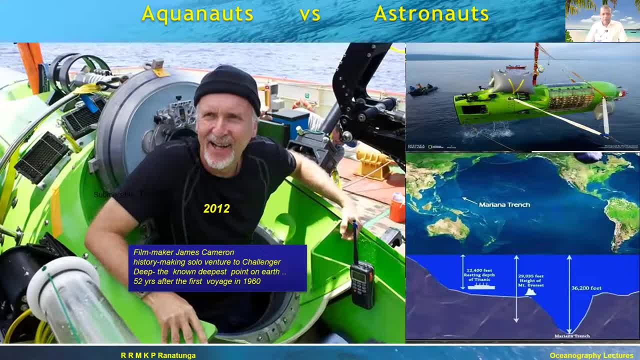 it's well-known filmmaker, especially the scientific people. fiction, right, uh, like the aliens, right. gladiator, right. the avatar, and then even the titanic was, uh, one of his great creations, right. so he's the one who went to be the deepest point in 2012. 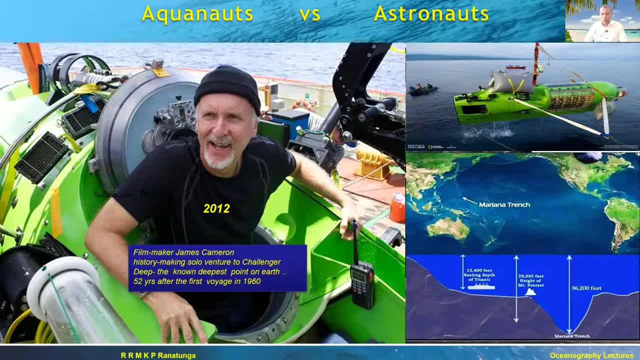 it is actually a solo venture. he went alone. no one was there, right, actually? um, you can see the, the, the submersible- we call it the submersible- where he used to go down right. so he has done a lot of like experiment. he had to control everything. 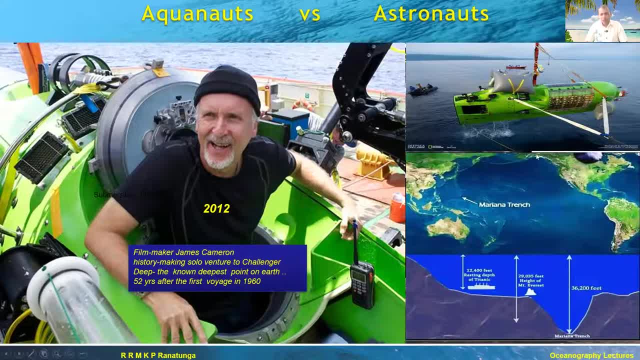 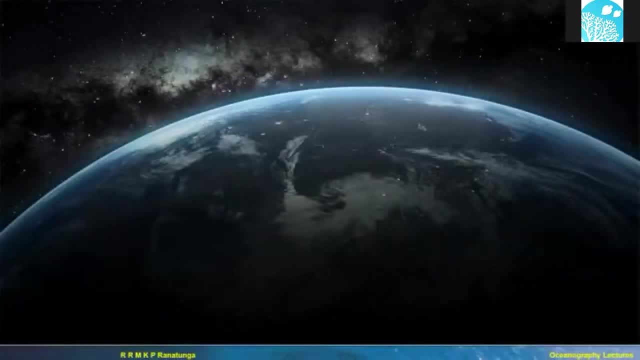 got even the samples and then- and he spent a lot of money on the not that expedition anyway- right, he never had to be making smartphones or evenuta or even stars or anything sleep category or any of the banana-type things that were going on in his life. 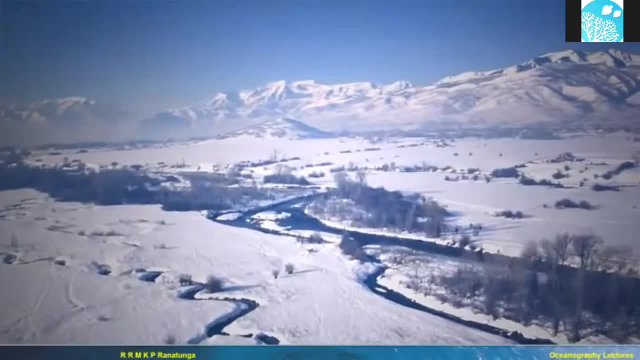 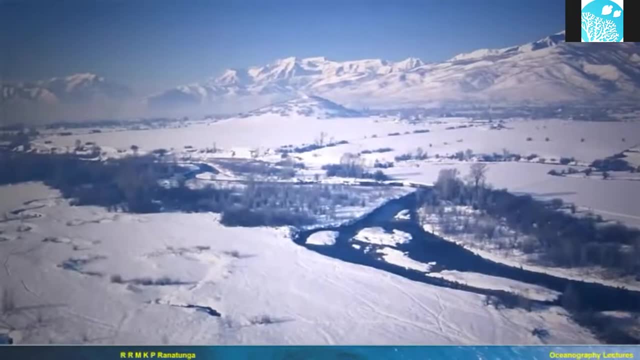 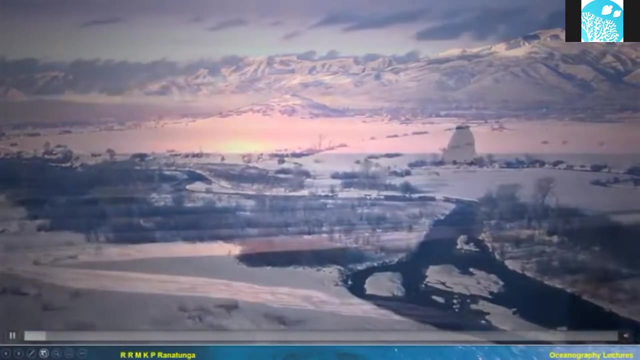 so he's all over. our brother joe's the only one dealing with that. but then we came to this history because he knew so much about human history after all those events about him dying before god, he had no idea how he was going to live our home. over the course of history, we've constantly learned more and more about 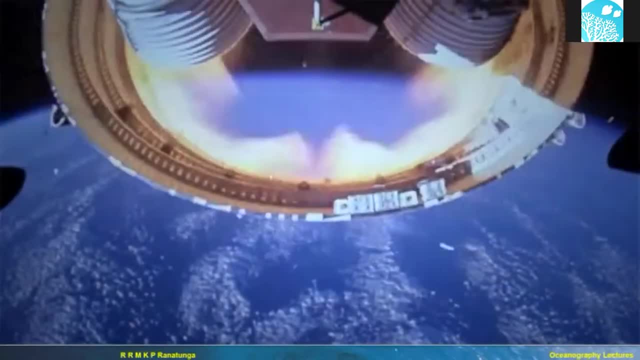 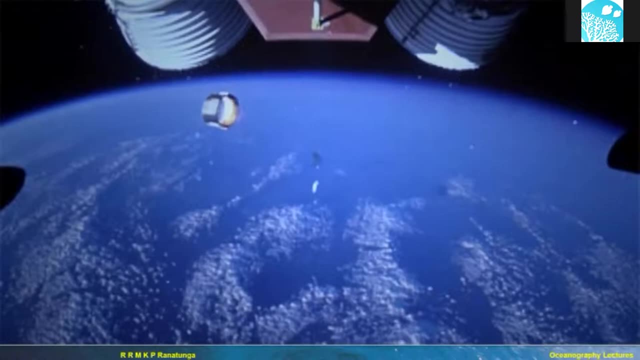 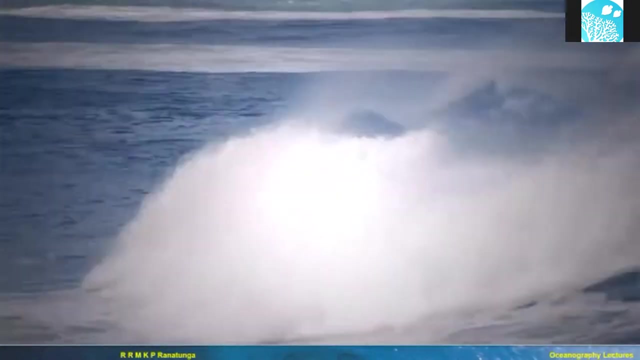 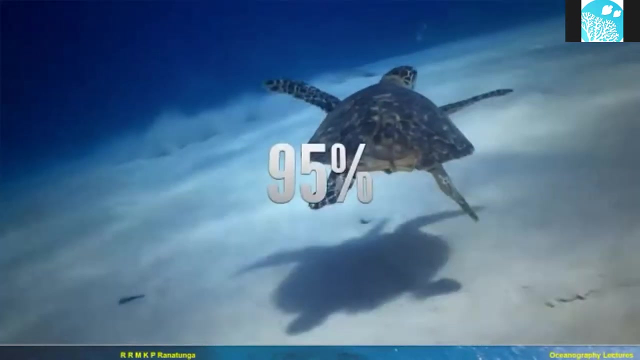 ventured beyond it. But there is one place, one place that remains a mystery, a place where darkness brings a new meaning to the world: the ocean. 72% of the earth's surface is covered by water, yet 95% of the world below the surface remains unexplored. We have better maps of Mars. 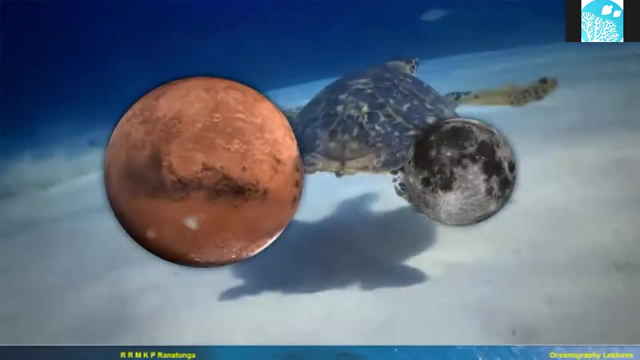 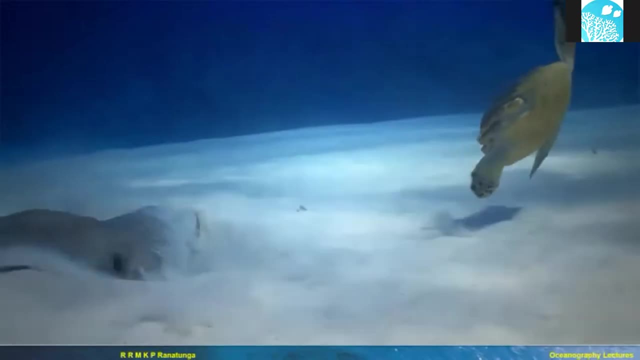 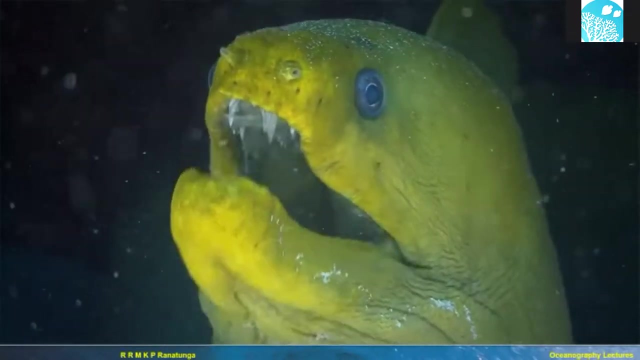 and the moon than we do of the ocean floor. Nearly 50% of all life on earth is also found in the ocean, But scientists estimate that at the very least a million more aquatic species has yet to be discovered, Which basically means that, theoretically, no matter how unlikely or 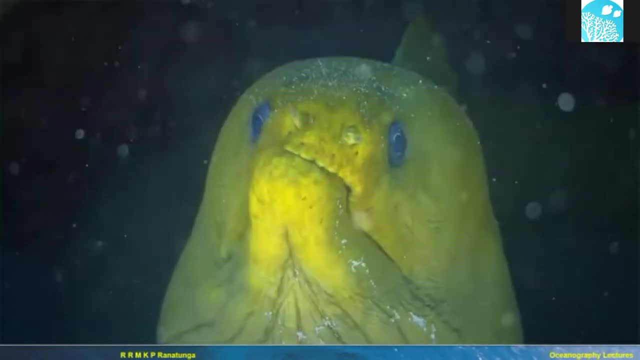 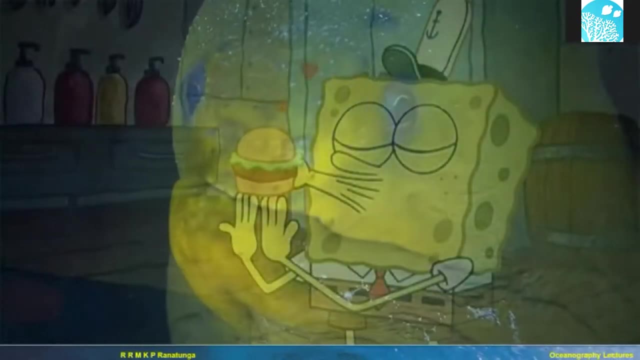 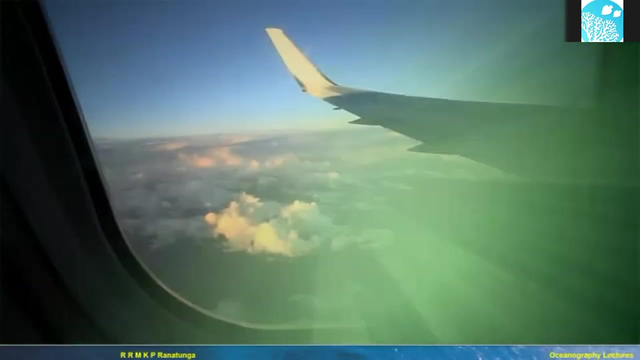 illogical it might be to us. now there is no way that we can discover the ocean floor. There is still a chance. a chance that a talking yellow sponge-like creature is enjoying a delicious Krabby Patty right as we speak. If you've ever flown with a commercial airline and tried to look out the window, 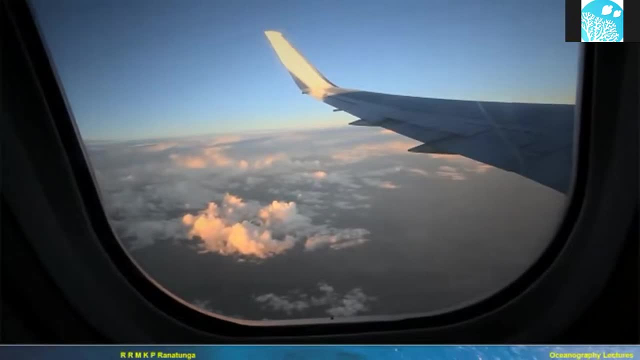 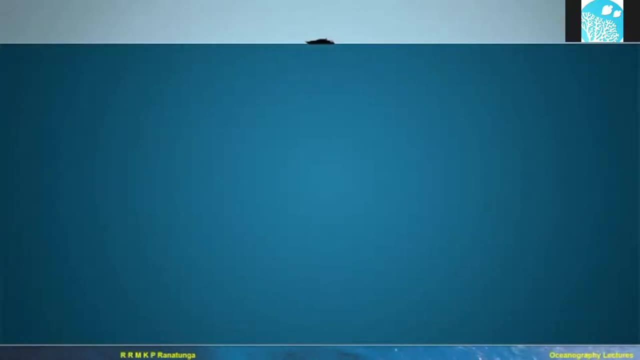 things will look pretty small, obviously, But keep that distance in mind. Now imagine that you're on a boat and, instead of seeing the ground from high up in the air, you see the ocean floor from the surface, how much your deep is. It's almost 11,000 meters. It's the lowest known point in the ocean. The most amazing thing, though, is that we have been there. Humans have actually touched the bottom of this place. And not only that: we did it in 1960.. 1960, that's over 50 years ago now- Humans would not visit again until 52. 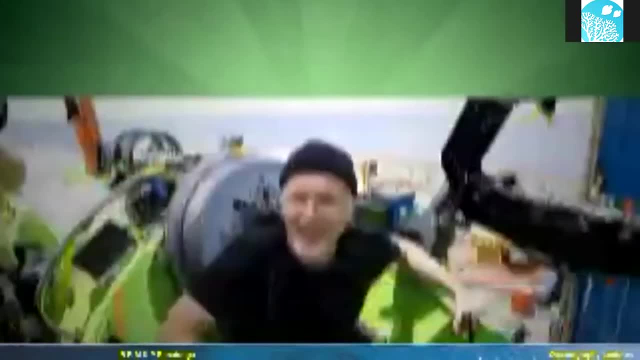 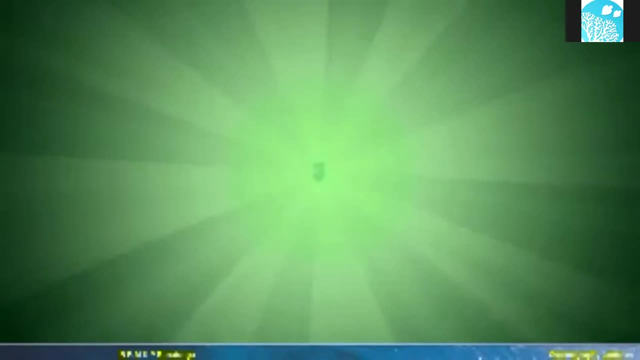 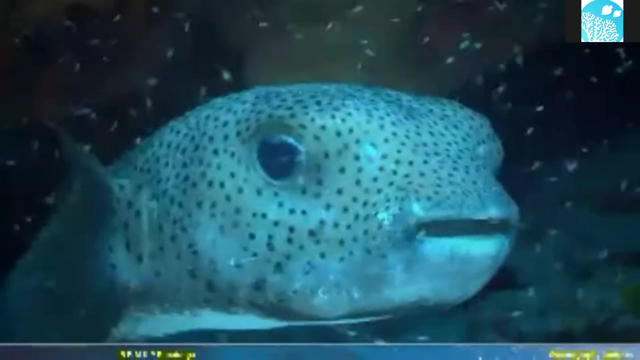 years later, when, in 2012,, James Cameron, the famous movie director, actually ventured down to the bottom himself. Marine animals have something called cleaning stations. At these stations, fish, sharks, turtles and other aquatic life congregate to be cleaned by smaller shrimp and fish-like. 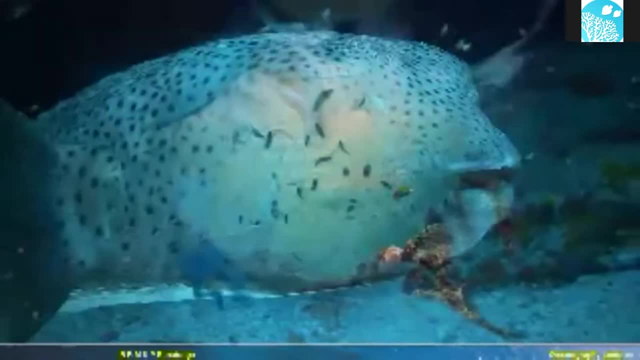 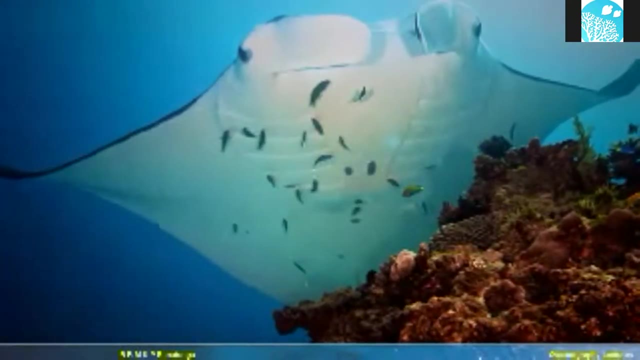 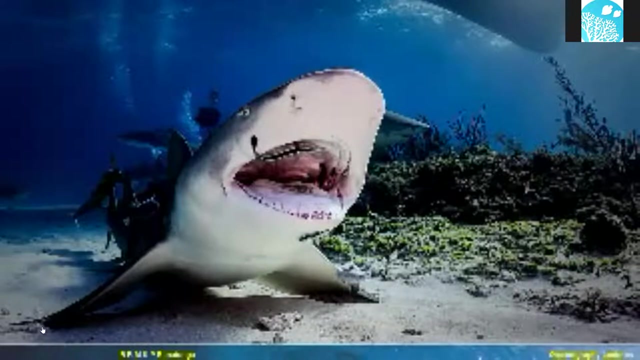 creatures. When the animal approaches the cleaning station, it will open its mouth and position its body in such a way as to signal that it needs cleaning. The cleaner fish will then remove and eat the parasites from the skin and even swim into the mouth and gills of any fish. 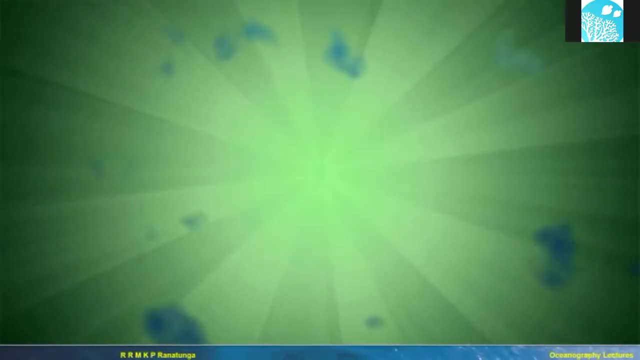 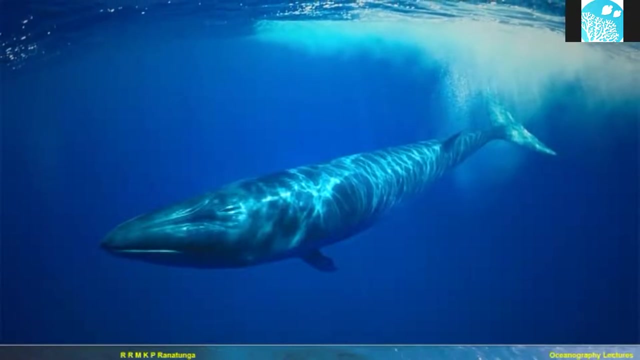 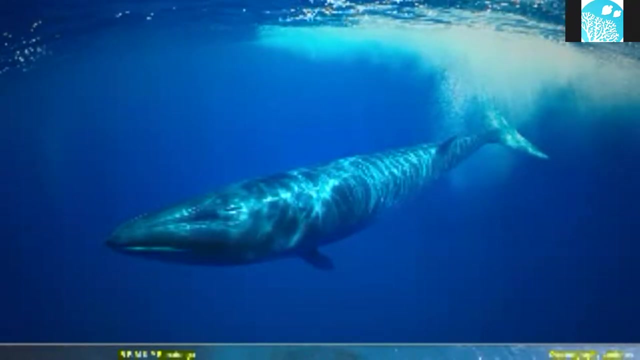 being cleaned. For decades now, scientists have been tracking a mysterious song heard in the depths of the ocean. The song-like sounds have been identified as belonging to a single male whale trying to communicate with others. The problem is that he produces sounds at a frequency of around 52 hertz, but most other 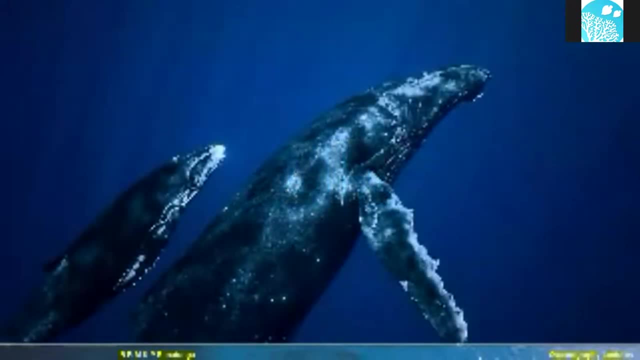 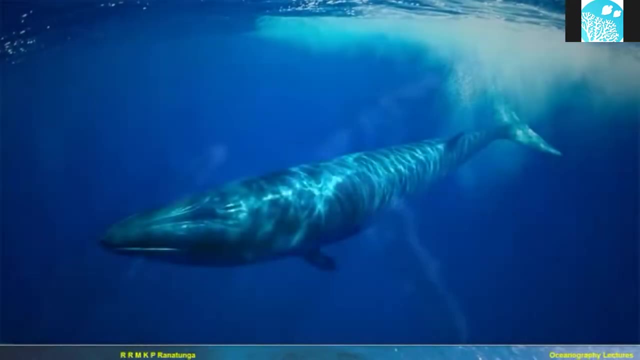 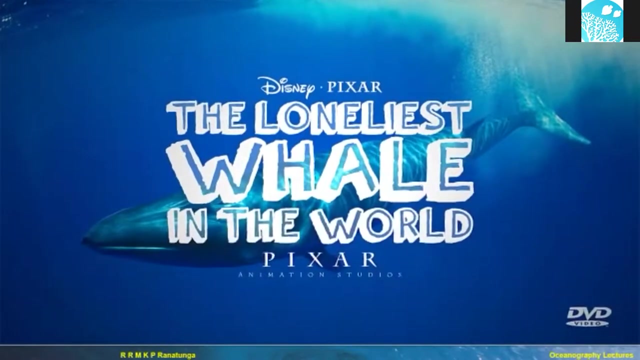 whale species sing at frequencies much lower, between the 15 and 25 hertz range. Thus his singing goes unnoticed, no matter how hard he tries. and it's been named the loneliest whale in the world, which, coincidentally, sounds like a perfect title for a Pixar movie. 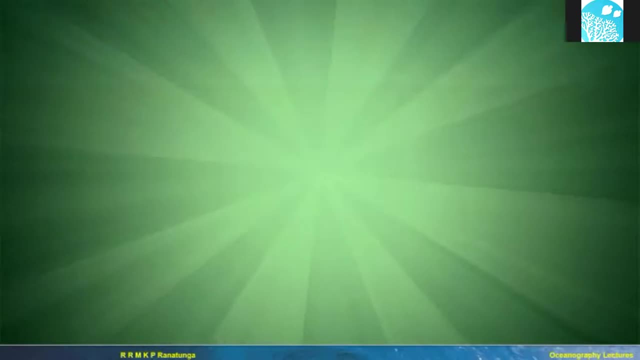 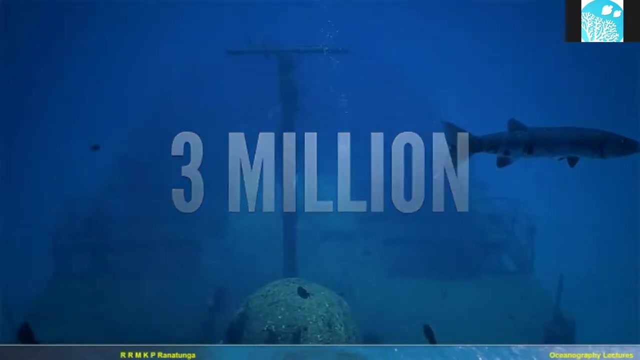 It's been estimated that roughly 3 million shipwrecks is right now resting at the ocean floor. As they slowly sank beneath the surface, never to be seen again, they carried with them all their cargo, their gold, everything. So, as we speak, there are several billions worth of treasures waiting to be found at 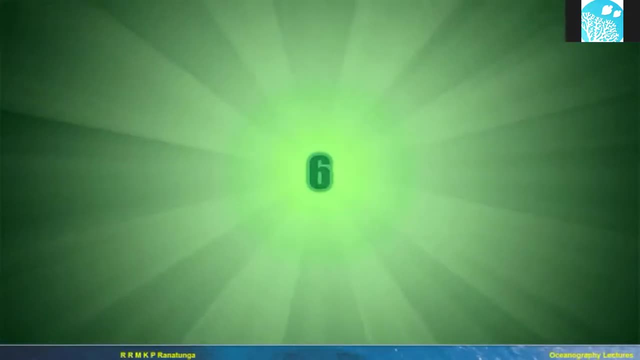 the bottom of the ocean. In 2012,, a video from an oil rig in the Gulf of Mexico spotted a highly unusual and surreal-looking whale. In 2012,, a video from an oil rig in the Gulf of Mexico spotted a highly unusual and surreal-looking whale. 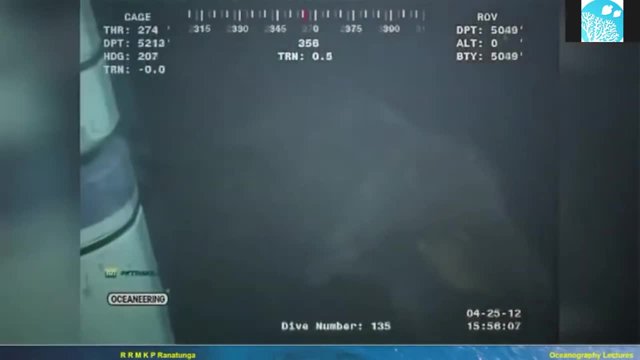 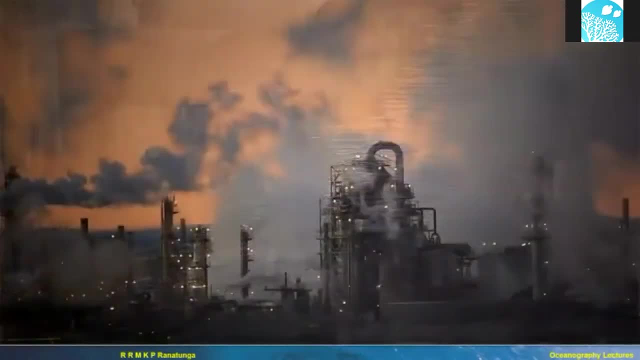 In 2013,, a video from an oil rig in the Gulf of Mexico spotted a highly unusual and surreal-looking whale. In 2013,, a video from an oil rig in the Gulf of Mexico spotted a highly unusual and surreal-looking whale. But let's not forget about our pollution of the skies. 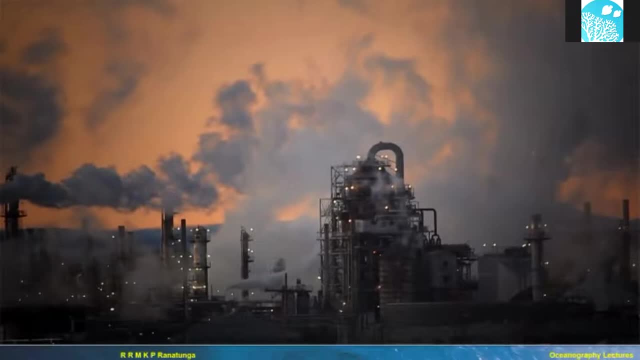 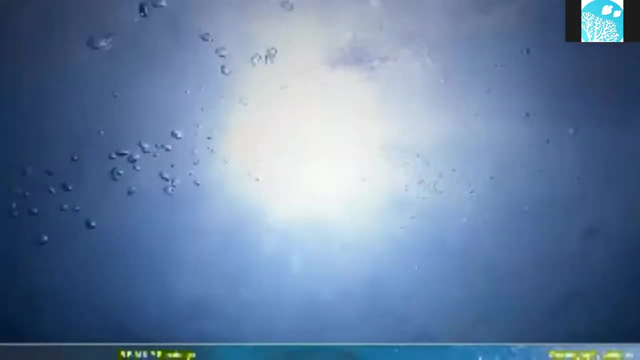 Global warming has an enormous effect on the oceans as well. About 30 to 40 percent of the carbon dioxide we release into the atmosphere dissolves into the ocean, rivers and lakes. It reacts with the water to form carbonic acid and starts a process called Ocean Acidification. 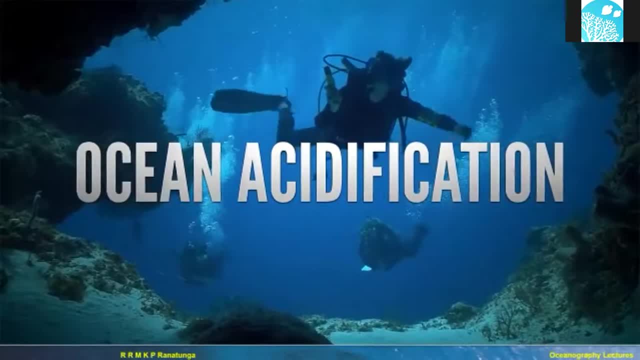 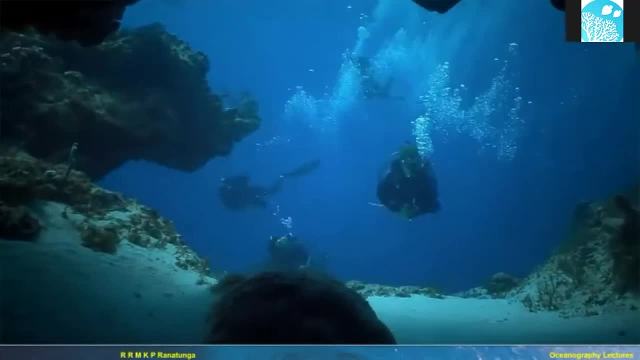 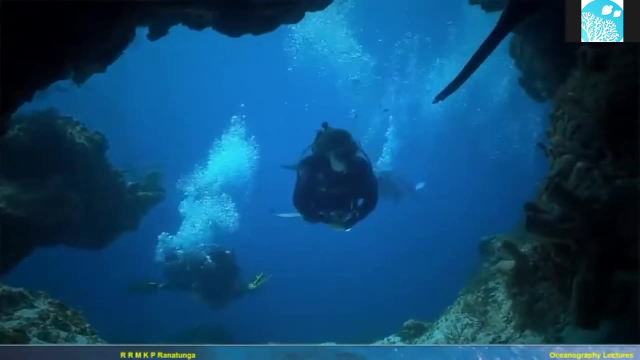 where slowly but increasingly turning our oceans into acid. Where slowly but increasingly turning our oceans into acid. Let me say that again just to let you know how moronic this really is. We are knowingly, knowingly, destroying something that is crucial to our survival and probably 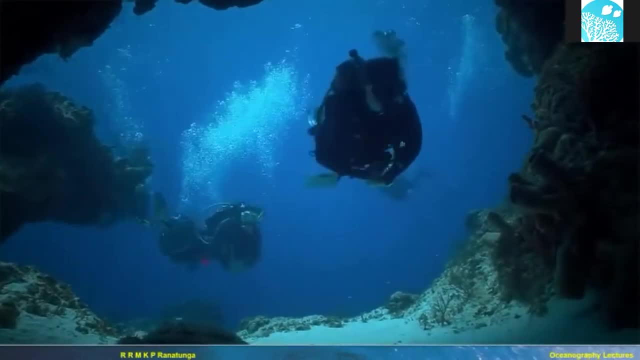 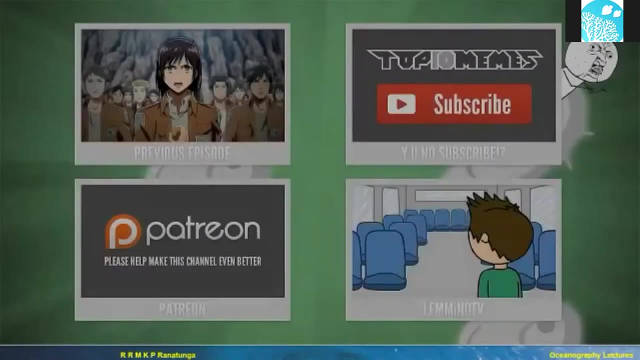 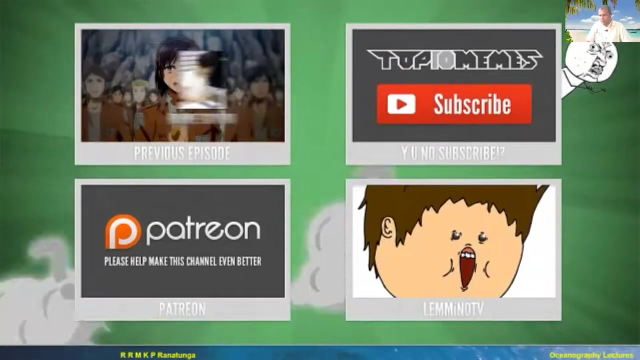 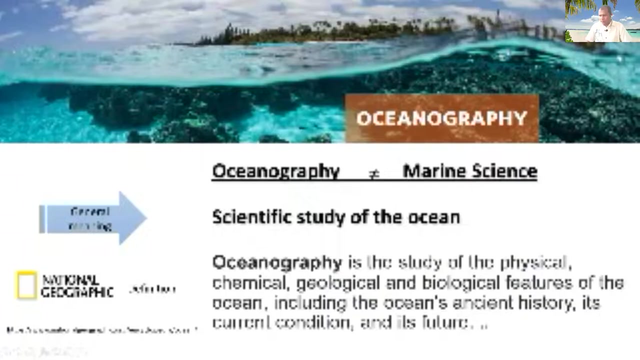 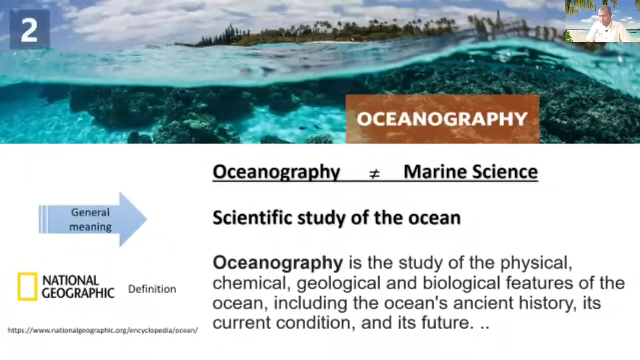 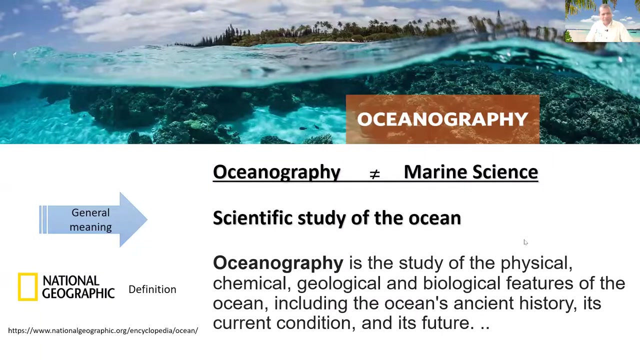 the reason we even exist in the first place by turning it into fucking acid Hari. I think you enjoyed that video. You can hear me. Yes, sir, Okay, So that video actually gave you some some sort of overall perspective or idea about. 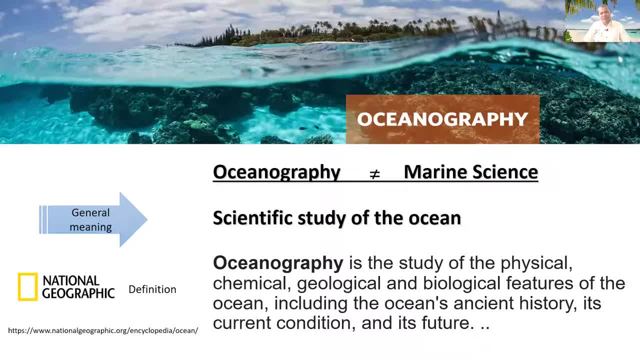 what I'm going to learn in this lecture series, right from the beauty of the ocean or its unique things with the ocean And, and as well as the the what is the situation with the ocean, the importance of the ocean, as well as the present situation and how the ocean would be in the future, that video gave. 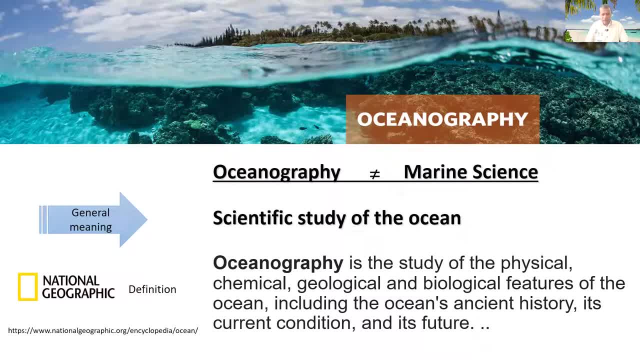 some sort of overall perspective, right? So oceanography- the term oceanography sometimes some people use as the marine science as well, But it's not the same thing. but I'll explain later on these terms not very wrong to call. 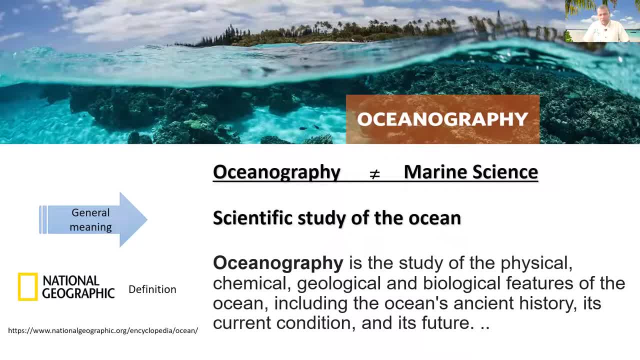 it as marine science as well as. but the marine science is a little bit more complicated than the oceanography. Oceanography is very clear what you learn in the ocean, but marine science is a little bit. there are more other things to combine, right. 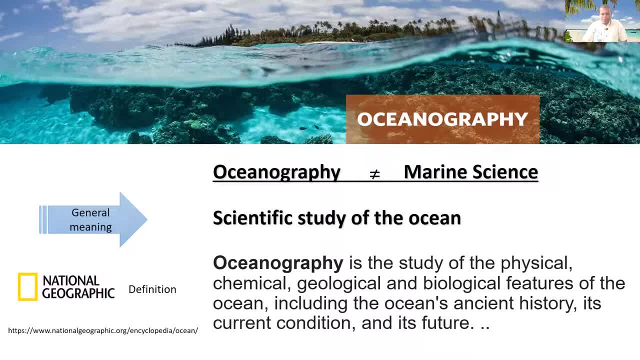 So, very simply, the oceanography is just scientifically simple. It's a scientific, scientific study of the ocean. but here we learn different aspects of the oceanography and then, together with the history and also the the present situation and as well as how would be the ocean in the future. that's what we're going to learn. 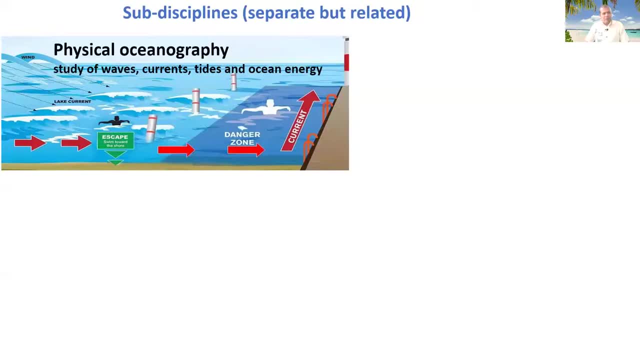 Basically the. there are four disciplines in the oceanography, four main disciplines. one of the discipline we call the physical oceanography- physical oceanography- where you will study about the waves, the tides, the currents and the the ocean energy, how. 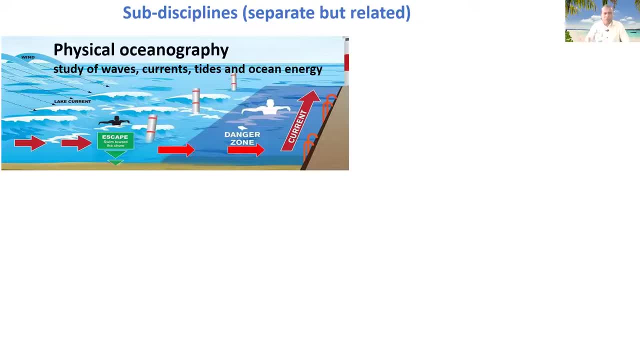 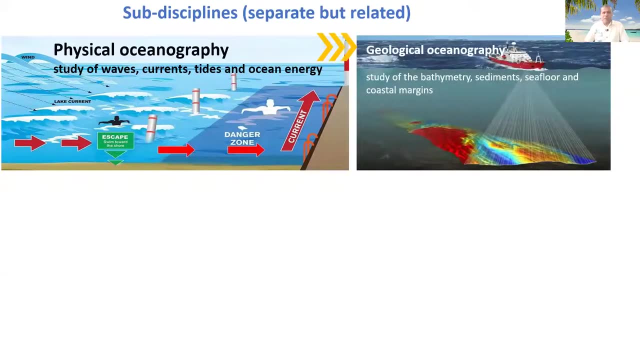 the ocean, water move, something like that, the physical features of the ocean, right. The next thing we'll learn: a little bit on the geological oceanography, like the how the ocean is formed and what is the content, What is in the bottom, what kind of things you can see there, and then how we can study. 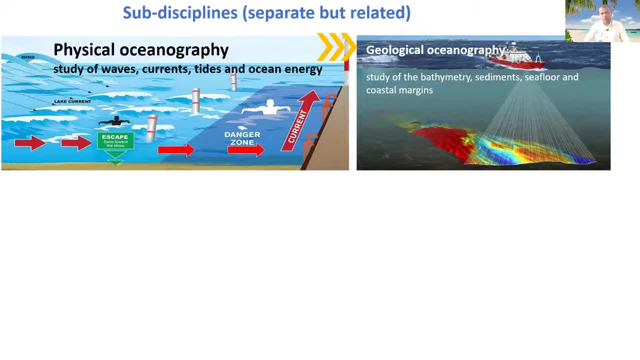 about then? what are the methods to study about the ocean bottom? because we can't see anything from the above or from the abode. but how are we going to study about the ocean? ocean flow, right. How it is formed, right. 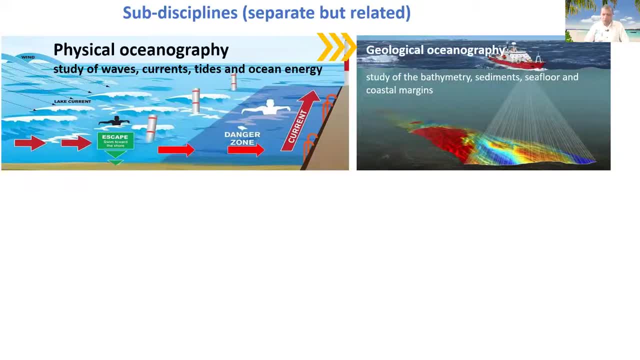 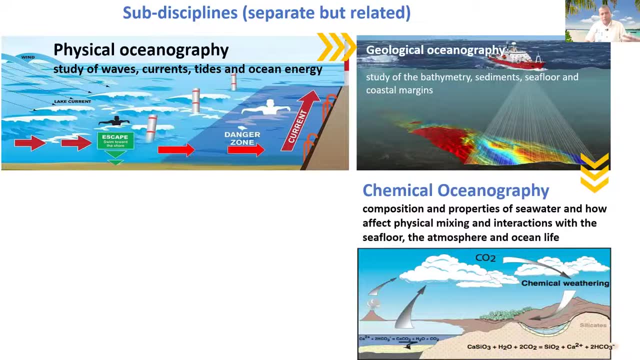 So this is, these are the things that you're going to learn in geological oceanography, And the third one is a chemical oceanography. Okay, Okay. So in the chemical oceanography, we will be talking about the, the, the ocean chemistry. 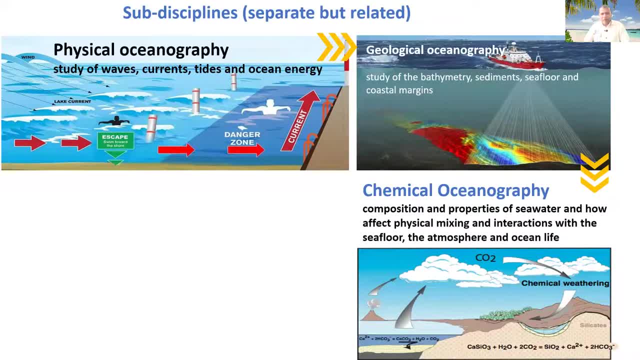 or the composition of a, and also the properties of seawater and how the seawater is moved and mixed. And then what are the chemical compounds or the how the seawater is formed, likewise, And the, particularly the, the ocean and land interaction and chemical interaction. something. 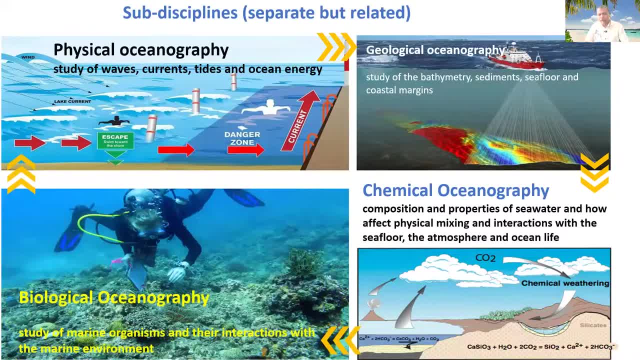 like that you're going to learn in the chemical oceanography. Finally, We will read all these- the physical oceanography, geological and chemical oceanography things with biological oceanography. That is the our main interest actually, here We are as biologists. we'll be more interested in the biological oceanography. 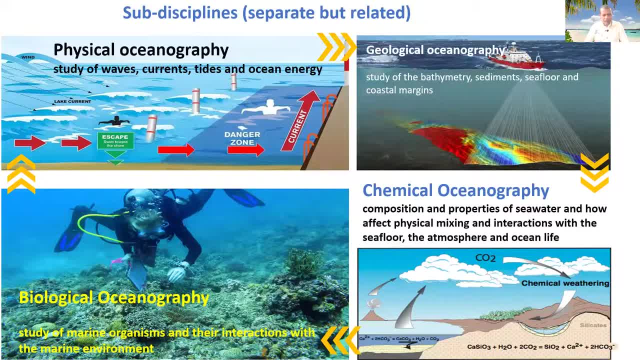 That's why we learn more about the, the animals, and how we, or rather the, the ocean animals, how they interact with the ocean in physical, chemical and geological. But as you can see, this is very introduction to the oceanography we will not cover very. 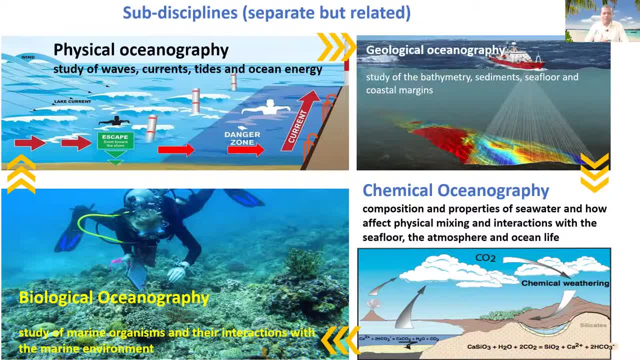 much on the biological oceanography, because in the second year and then of another, especially if you are doing special degrees, we'll talk more about the biological aspect. So this lecture series will more look at the physical, geological, chemical oceanography and then a little bit of biology as well. 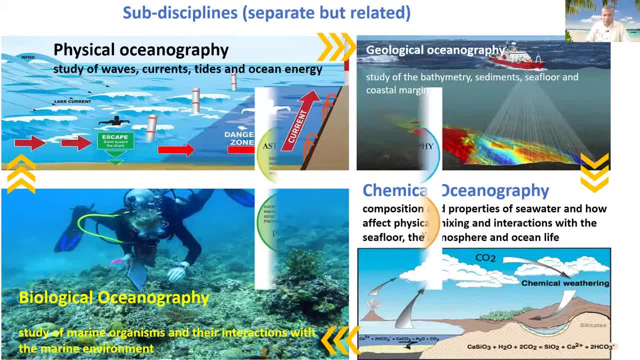 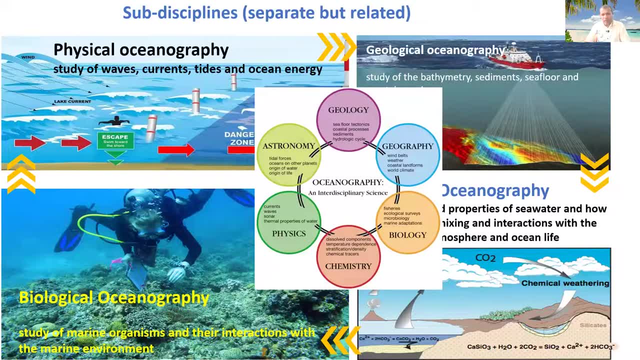 Right. So that's how things are organized and and it the subject. actually, it's not only these disciplines, but there are so many other, like even the astronomy, perhaps, right, geography, And it's a combination of all these subjects. 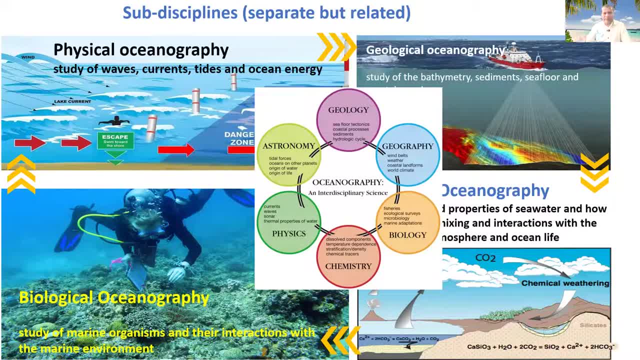 And that's why we call this subject as a interdisciplinary subject. It's also a multidisciplinary because it's involved a lot of areas, And it's interdisciplinary means they are all depend each other right. So we need to know biology, chemistry, physics, geography, geology, perhaps sometimes astronomy. 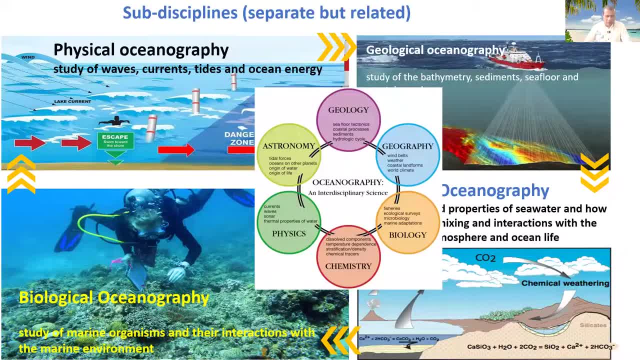 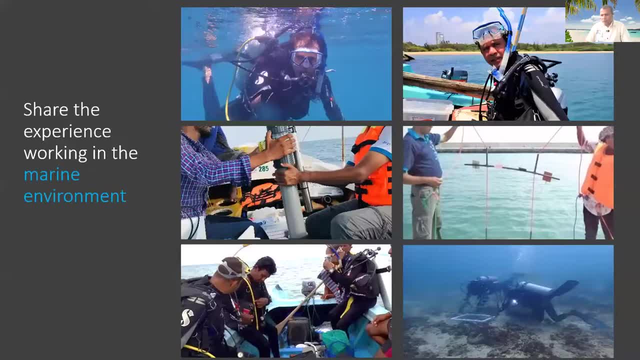 Thank you, Thank you, Thank you. So, since we have discussed some of the things last week as well. So I have a lot of experience in working in the marine environment doing research, And also we're working a lot on the environmental impact assessment from quite a substantial 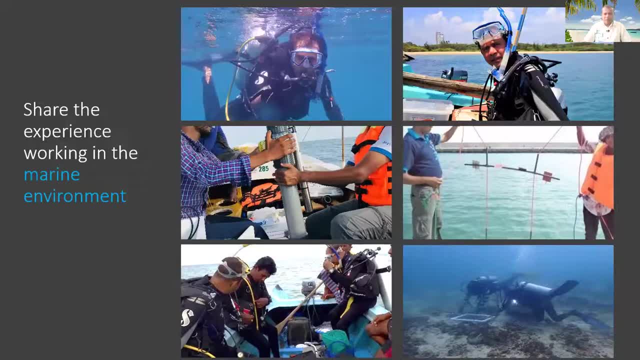 existing as a less planned projects. Okay, if you're going to make a new port or a harbor, we have to do an environmental or we have to get an environmental clearance. we call EIA or otherwise, Environmental Impact Assessment. To get this one, we need to do some surveys. 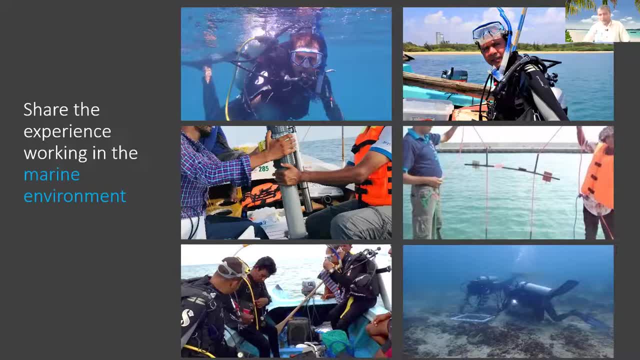 Doing this, we have gained a lot of experience about the marine environment around the country, So definitely I would be able to share with all- not all- at least some of these things right, Which we will discuss over the time right. 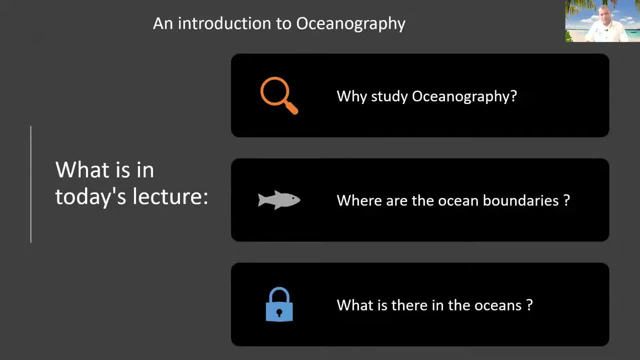 And in today's lecture. right Well, I'm just trying to give you an understanding or a very brief introduction, not to give too many things in the very first couple of weeks, but at least I'll I'll be discussing the few things. 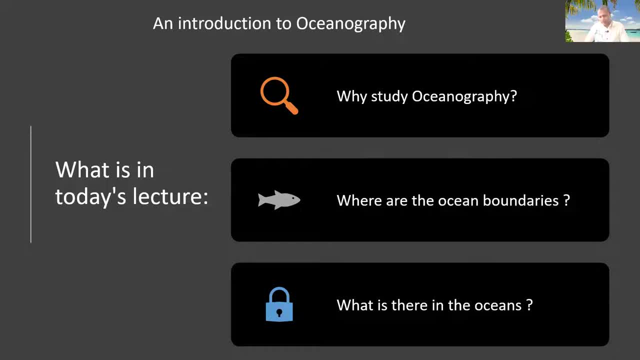 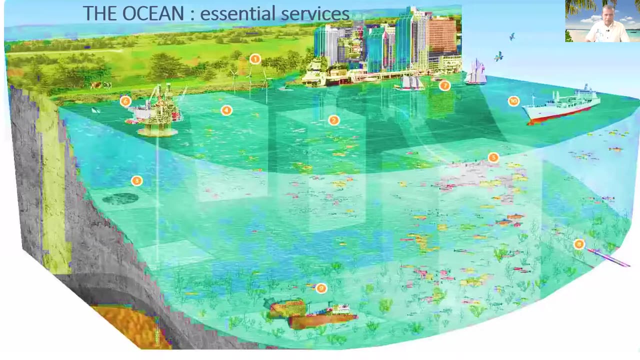 like: why study oceanography If I don't think you have time to go to the next section? that's where the boundaries of the ocean. But let's see why we should learn oceanography as a subject, right? So let me show you this. 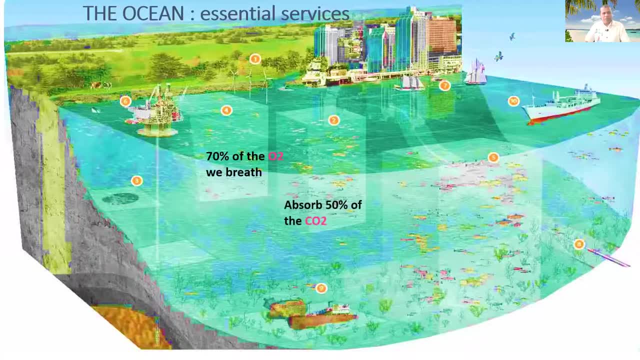 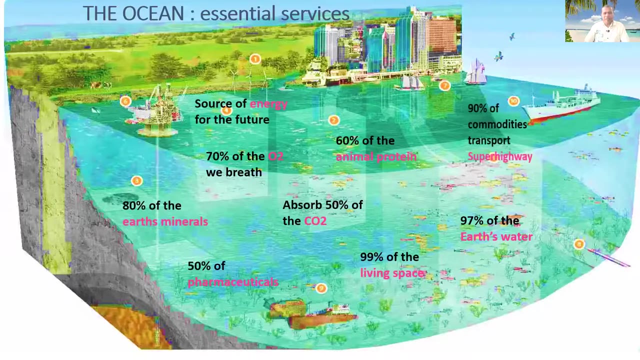 I can see the 70% of the oxygen produced in this ocean and more than half of it is oxygen, half of the carbon dioxide that produces soap in the ocean and it's 90% of the living space and 97% of the earth's water in the ocean and 60% of the animal protein come from the ocean. 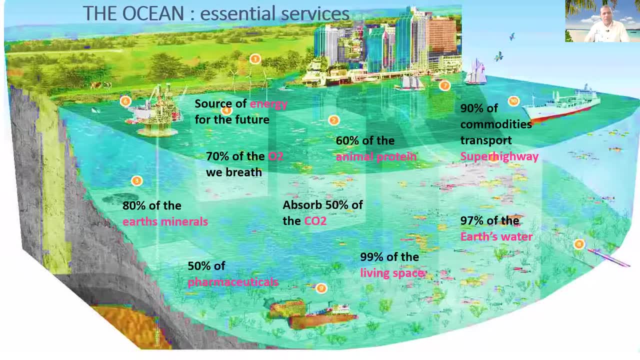 and its source of energy right, and it's a future resource base of the lot of minerals. and you can get a lot of minerals from the ocean. even there, in the terrestrial environment. there are even the. we can extract a lot of pharmaceutical products from the ocean. and not only that: 90% of the 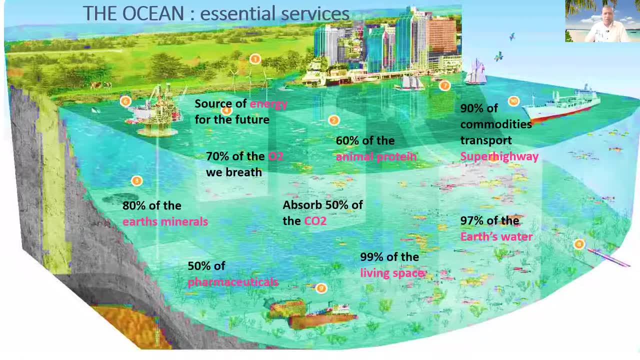 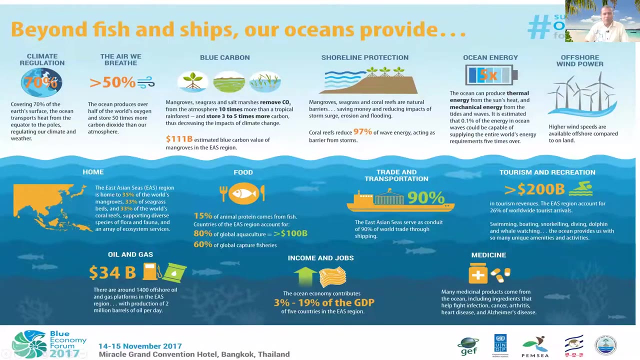 commodities like the goods, are transported in the ocean, and we call the ocean as the super highway, right? so these are some of the things that the ocean provide for us, but that's not all right, as you can see in these, with what we call the infographics- right, there's some graphic as well as information. so these kind 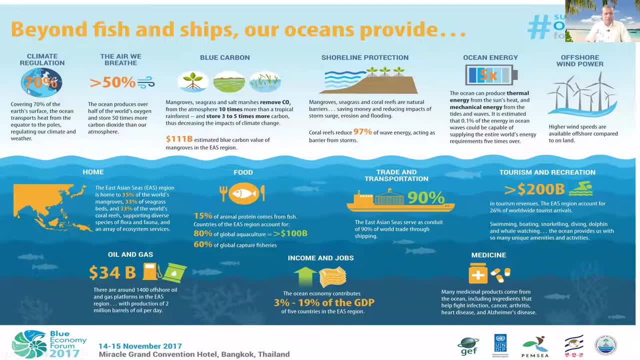 of things we call the infographics right, so it explain everything, from how much the ocean will contribute to the climate regulation, right, the the weather that we experience today is very much controlled by the ocean and you might have you know that even the like any like low pressure shown. 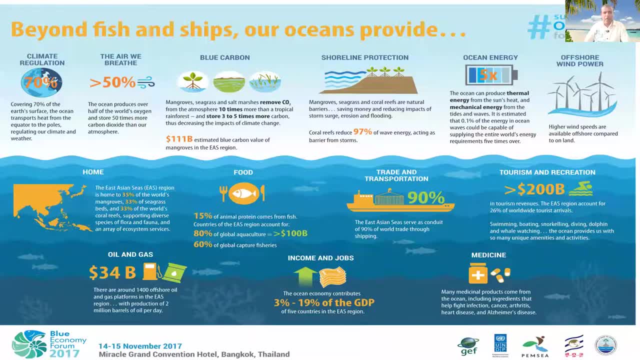 in the ocean, triggering some of the, the cyclones, likewise a lot of things in the, the terrestrial environment, or that we are experiencing. they actually, uh, coming from the or the regulated by the ocean, and even the. the air we breathe come from the ocean and we talk about the blue carbon, that, that the, the ocean store a lot of. 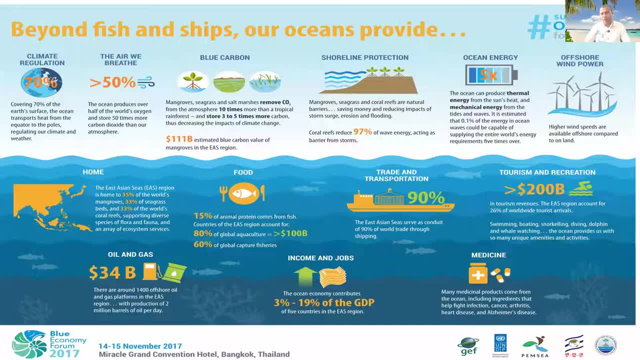 carbon dioxide and inform carbon in form of carbon dioxide- we will discuss this in later- and from shoreline protection and the the energy right, this lot of energy in the ocean, if you can extract that energy right. even here mentioned that, if we can extract one percent of the energy that we have in the ocean. 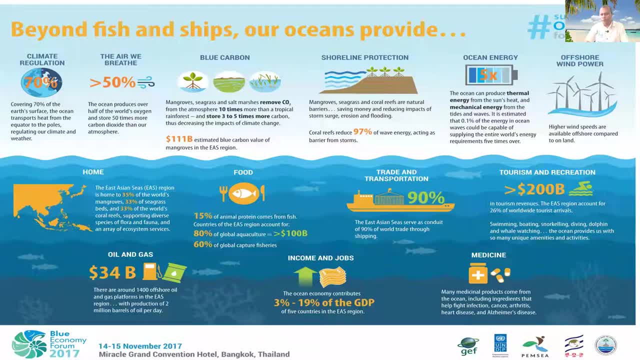 that's more than enough to provide the power to the whole world. right, you can imagine how much power power is in the ocean, but we are not really extracting this and we even the offshore wind power- we can have a wind power station, and and also the ocean is the habitat for a lot of. 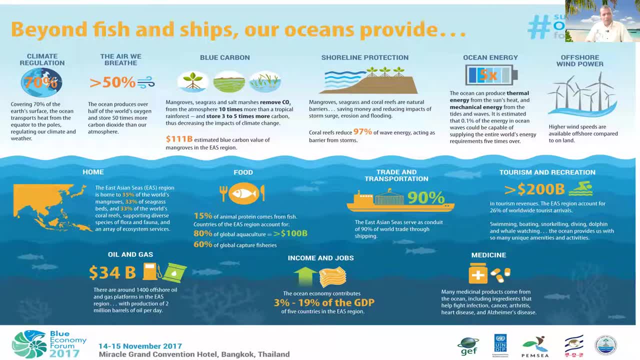 important habitats like the, the mangroves, the seagrass pits, the coral reefs- one of the most important ecosystems in the planet. right, so these are in the, the ocean, and how much food that the ocean is provide for us, and how many people live on the ocean, and and the other thing. 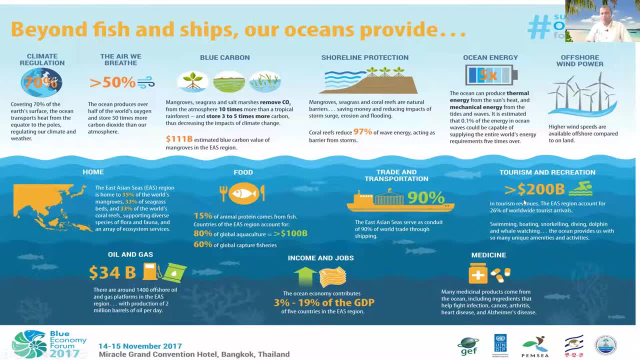 is the transportation of goods and tourism and recreation right. very much the tourism is depend on the, the, the ocean- in particular countries like treeland right- and the oil and gas. there are a lot of oil and gas producing in the ocean, what you call the offshore oil. 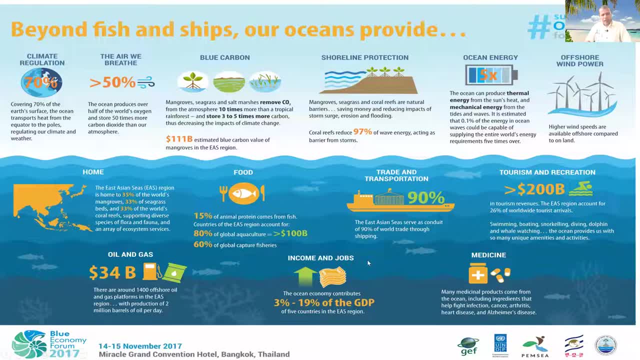 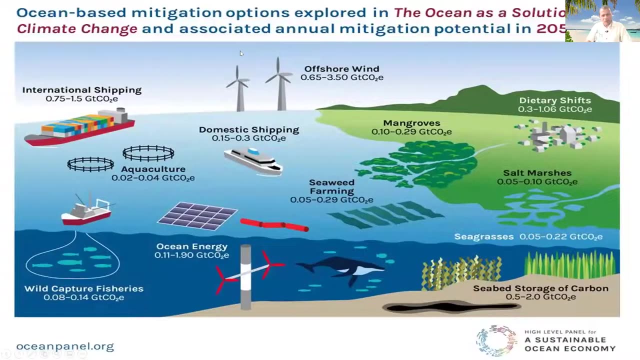 um platforms right, and the income and jobs and medicine. likewise, there are so many things that we can get from the ocean, but we talk very little about the ocean right. on the other hand, now the scientists believe that the ocean is the most important place, like we are talking about now. that 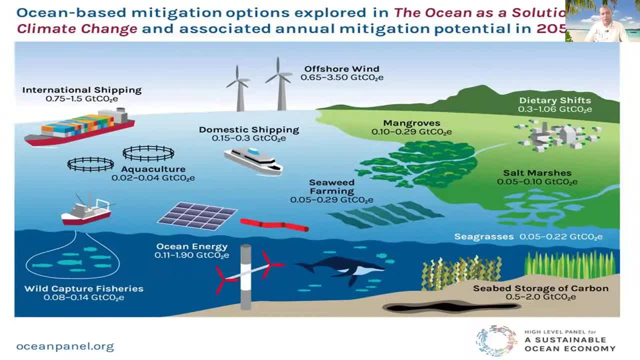 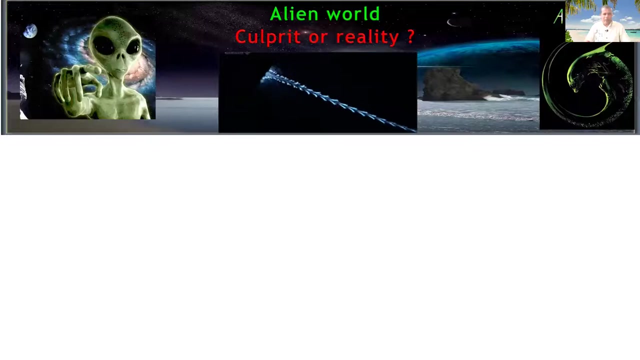 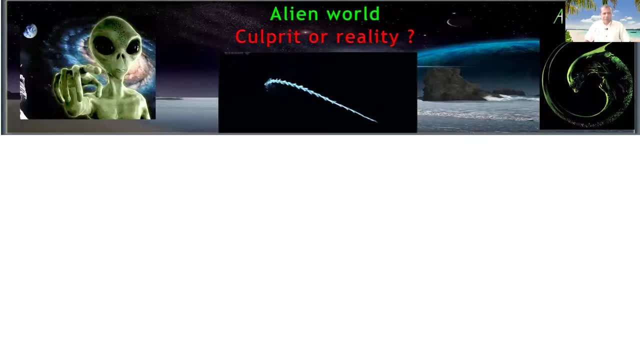 like we talk about this alien, like we talk about this alien species, right. you might have seen even the movies the aliens, right, but this term aliens- are they a culprit or really make a mitya a culprit, or really make a mitya, right? just look at the ocean buttons, right. these are some of the images of the animals living in. 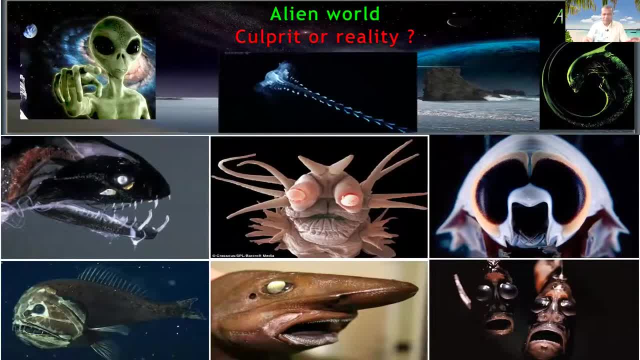 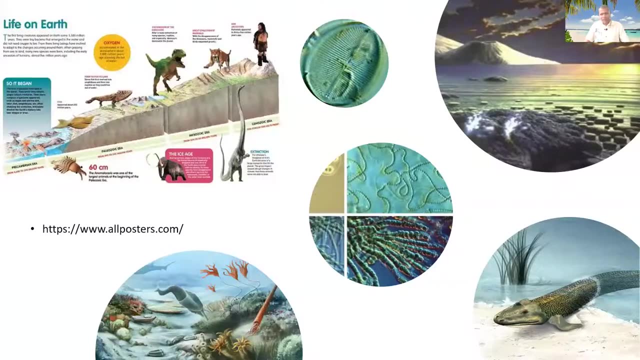 the ocean. you can see they are. they looks very weird, right, so just like you can call them as aliens, right? just few images, but there are a lot more fish or other marine organisms. just look like alien, right um. another more important, most important thing is that the, as we heard, or as we know, 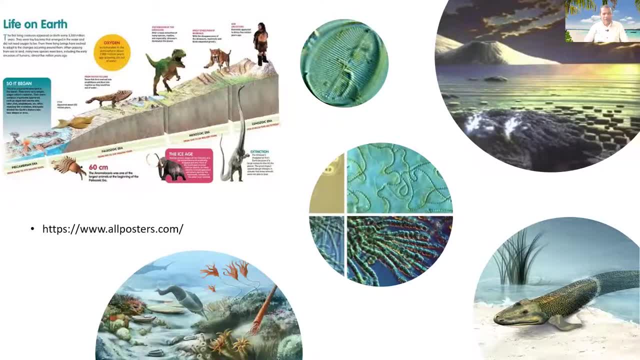 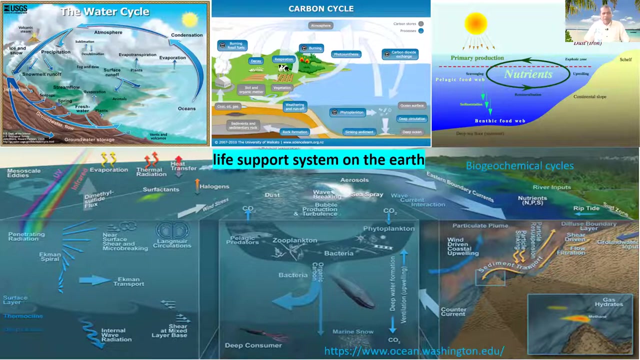 the life began in the ocean. the life began in the ocean. the life began in the ocean. so it's very important to know that, how we descend from that prehistoric creatures, from today's right and other very important thing is that the water cycle, the carbon cycle, the nutrient cycle and all the other biogeological cycles that the 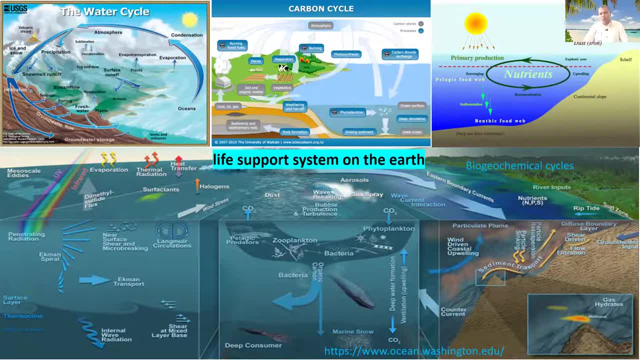 we have on our earth, they all controlled by the ocean. right, the? the ocean provides you all the the the basic things for the cycles to run, and that's why we call the ocean as our life support system. right, the? the ocean is the earth's life support system, just like the our heart. 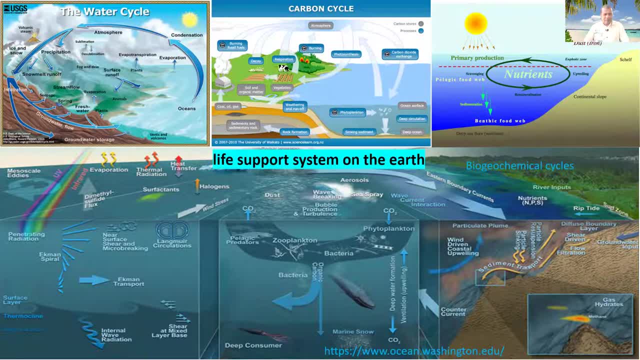 and the lungs in our, in our body, right. so it's the lifestyle system, right? if? if something wrongs, if something goes wrong with this life support system, the whole earth is going to collapse, right? so that's where the the importance, right? so, um, why the ocean is that important? 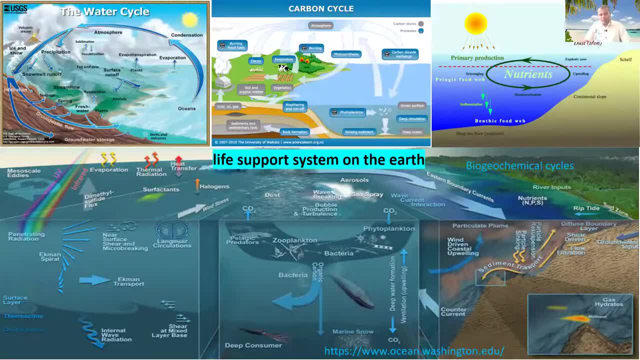 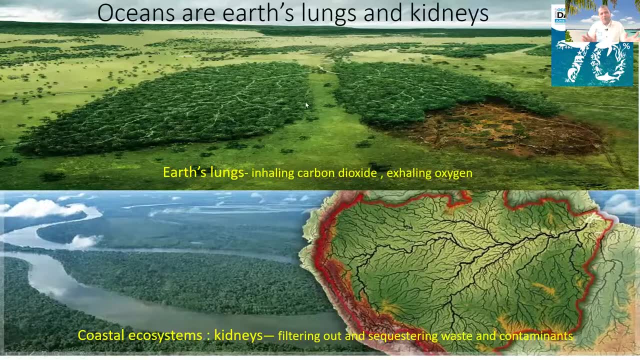 for everybody, right, and even the existence of the earth, right. and this, the two images you just look at: the, the, the, the oceans, in particular the coastal ecosystems and also some coral reef, seagulls, but they're like the earth's lungs, but these lungs, usually the lungs, take oxygen and exhale the carbon dioxide. 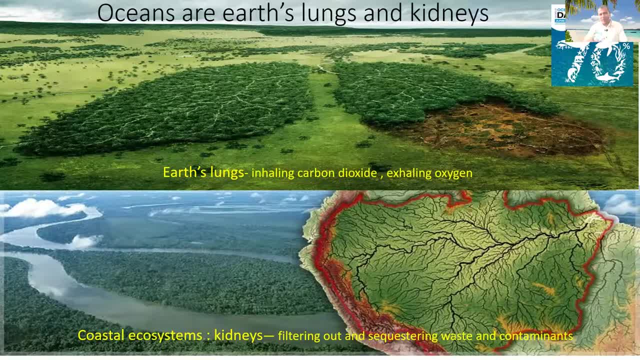 they inhale oxygen and exhale carbon dioxide. but these lungs, they absorb carbon dioxide and right exhale oxygens, very. that's the oxygen that produce, that's the oxygen that will breathe right. at the same time, they are the like kidneys, like filtering out the most toxic substances and in any other contaminants, in particular the 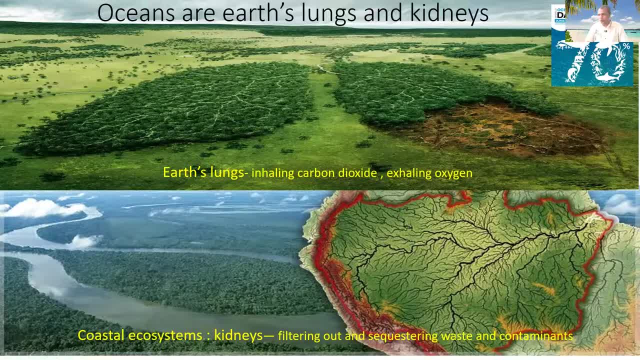 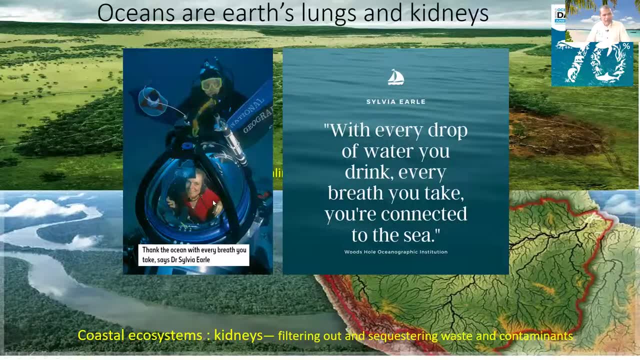 coastal ecosystem right. so i don't know. anyone of you have heard about a woman or the lady or legendary um a person called dr sylvia earl. i don't even know dr sylvia. any right, other military, impossible right. you can search in the google or anywhere about dr sylvia. 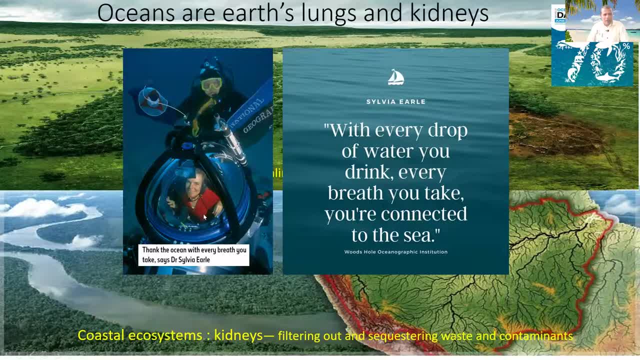 earth right, one of the uh, one of the living right, legendary ocean explorers. i see, though, she's a woman. she has been a like a led, one of the uh like uh aquanauts doing a lot of exploration in the ocean, including even like working in the submersible. um, there are a lot of inspirational. 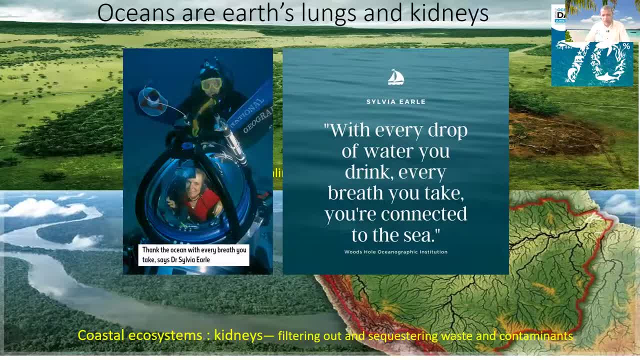 talks given by her. like we will give you the scrolls, uh uh, there's marea that's working to. like you can search and you know i can. later on i'll show you some of the her talks. like, as you can see, with every drop of water you drink, every breath you take, you are connected to the ocean. 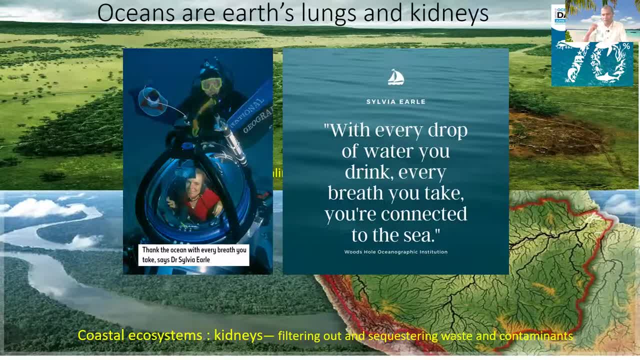 right. so there is no exception. right from every drop of water and every breath that you take, you are connected to the ocean, which means we all connected to the ocean, though we are. like we consider the ocean is like disconnected. that's why we're right, if you understand the ocean right. 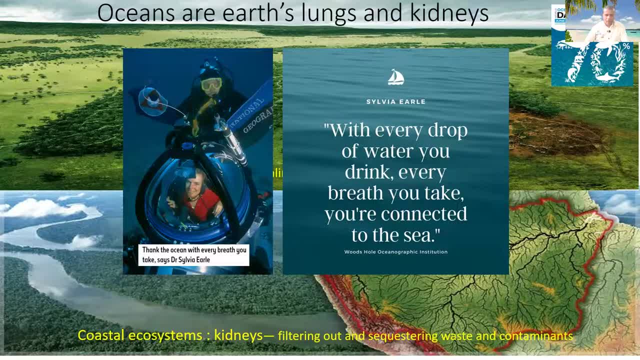 you connect to the ocean. you are connected to the ocean with the ocean. right, none of us do anything harm to the ocean because that much we are connected to the ocean in many different ways. right, and we as sri lankans, how important the ocean for us. 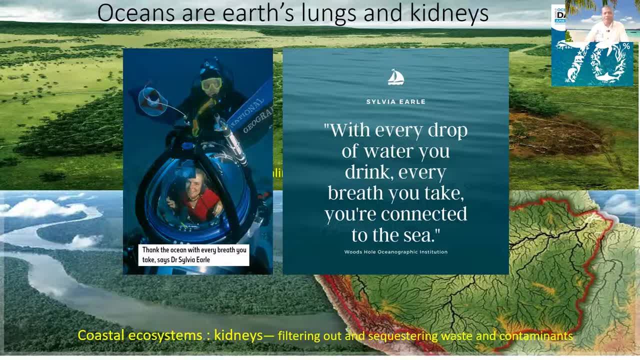 right, especially since we are an island nation. right, we are surrounded by the ocean and then we are small island nation, but we have a big ocean area with a lot of resources. but do we really get maximum out of this ocean? that's something we have to discuss in the future, right? 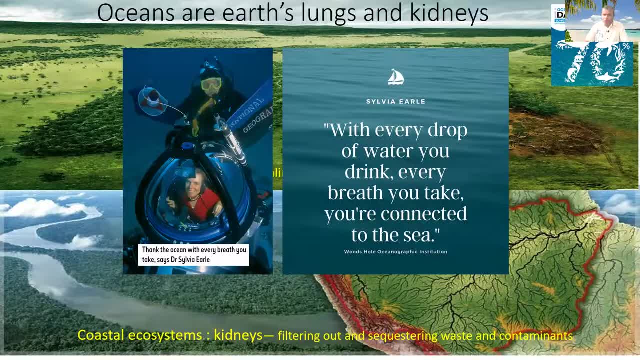 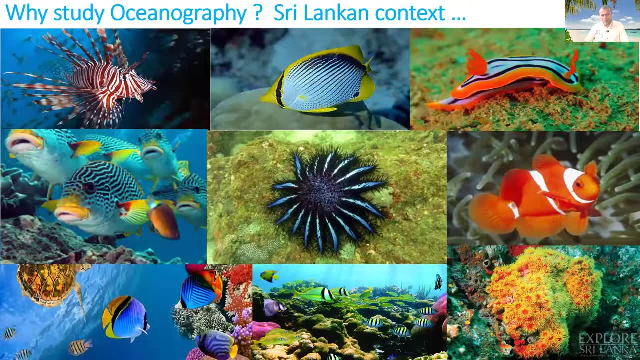 but other than that, how important the ocean is to us, especially the, the biodiversity in the ocean. right you can see these beautiful images of the ocean, of our oceans. right you can see these beautiful creatures, very colorful animals, and one of the reasons why the ocean is interested for many people, for like underwater photography or 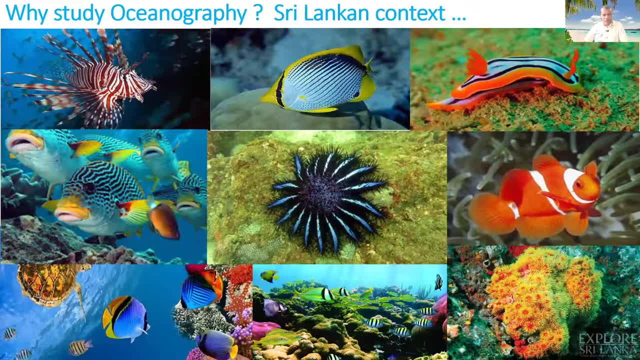 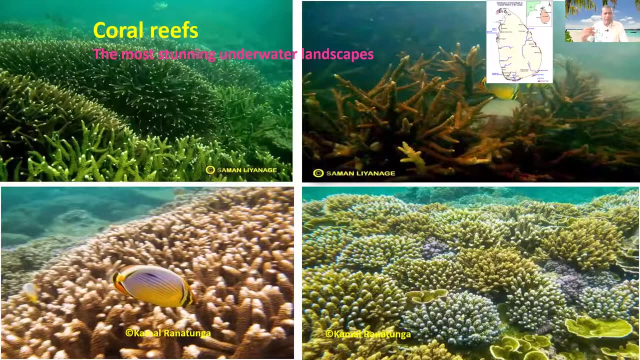 filmmaking, because it's the beauty, the colors, so much of colors in the ocean, even then the, the terrestrial environment, right, and and from this, the fascinating coral reefs. we call the the most stunning, almost fascinating underwater landscapes. right, there is no any other habitat that could be very colorful or diverse as a coral. 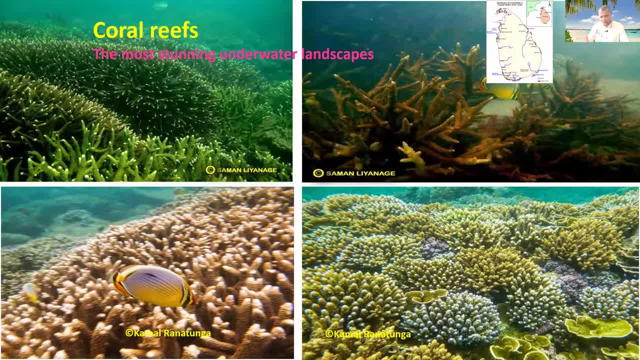 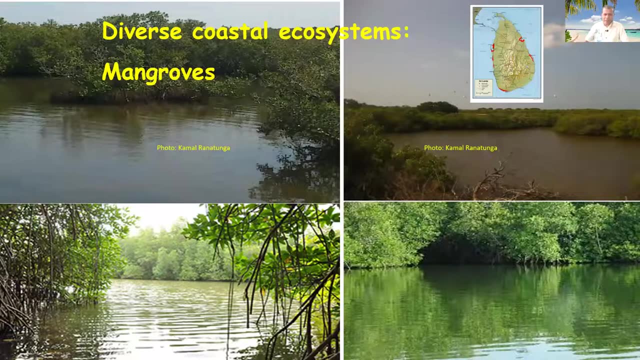 as you can see from some of these images- they all some of my own images and for that to this, the coastal ecosystems, particularly the lagoons, estuaries, right and and which support the mangrove ecosystems- very important ecosystem particularly they absorb a lot of carbon and also these mangrove habitats- is a 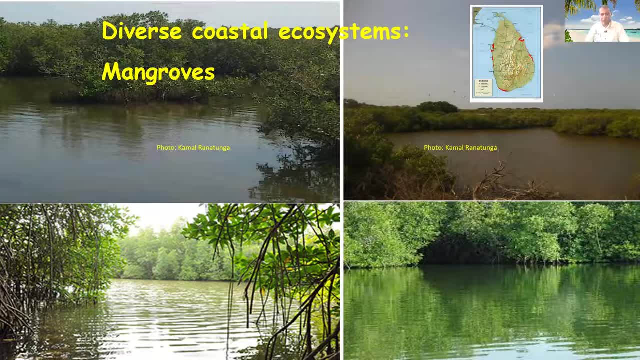 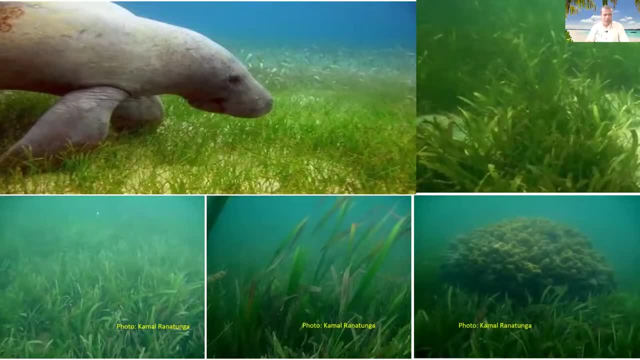 habitat for a lot of larval stages of fish, prawns, crabs and lot of economically important fish species. have right and the seagrass bits. I think you might have not even seen this seagrass bits, though. they are very common, especially even in the lagoons. 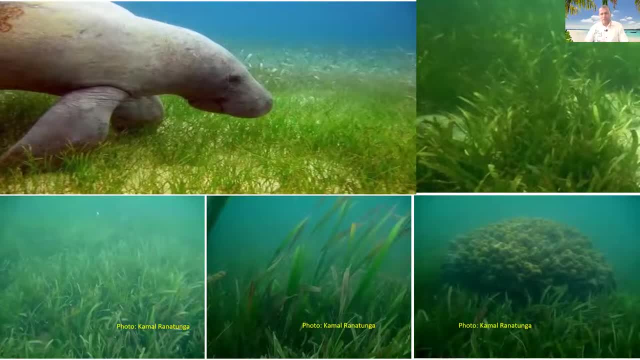 but you might not have a chance to see seagrass bits where they even these gilgons, where they live, right. this bottom image is actually I took in Jaffna Lagoon where there was beautiful seagrass bits in very shallow waters even right there, right, you can't like you see like it's like a grassland when you go, when you're snorkeling in a. 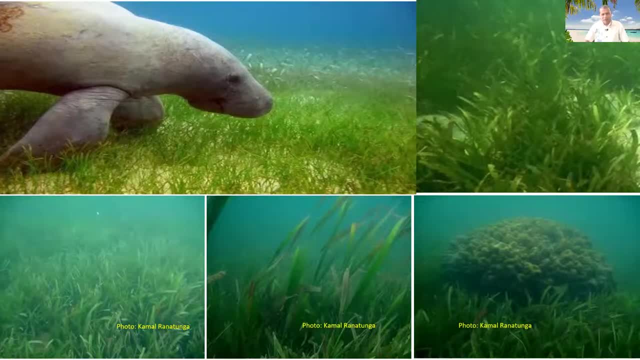 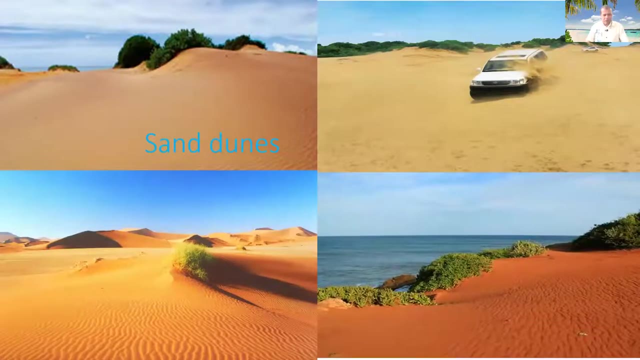 seagrass bit. it's just like you are in a grassland. such a beautiful environment with a lot of marine habitat, marine organisms as well, right. and from that to this, the sand dunes: right, you might have seen this. all these actual images from Sri Lankan sand dunes. 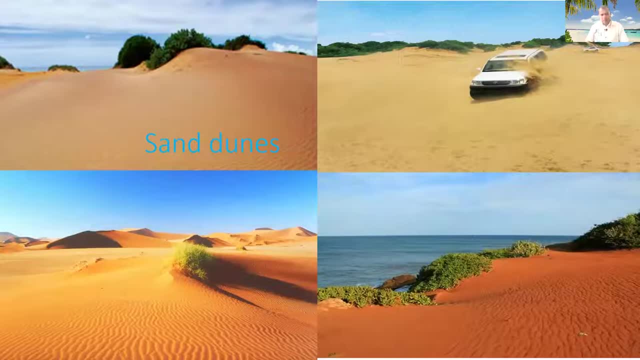 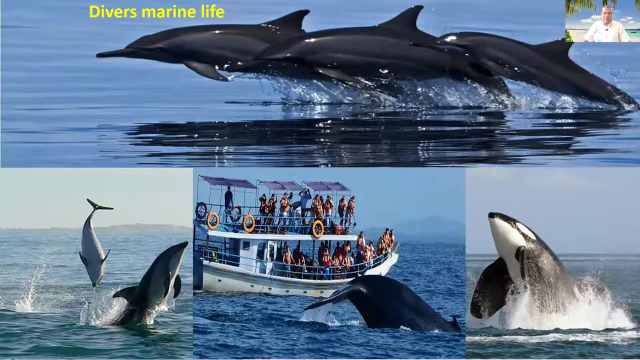 very interesting. some are in Boondallam, another unique ecosystem. there are unique plants and animal life in the sand dunes as well. right, and the other important thing is this: marine life, the marine mammals in particular, right from dolphins to whales, there are more than 30 species of marine mammals just out in the ocean. 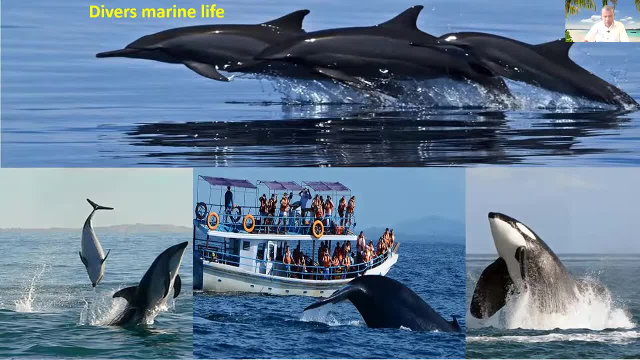 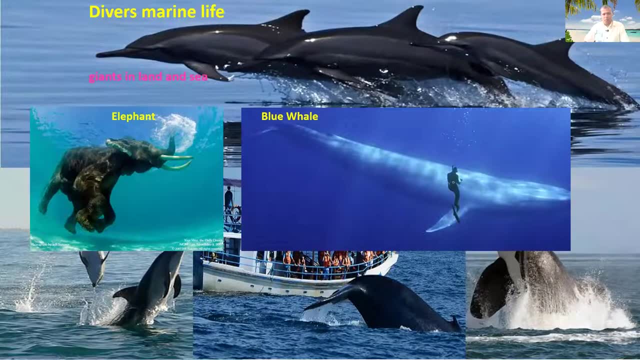 right and, most importantly, right. so I don't know anyone of you ever heard about this one like or ever thought of this one. the Sri Lanka is is perhaps the only the country in the world where you can see the terrestrial giant that is the elephant and the blue whale, the largest animal on our planet. right, both terrestrial one. 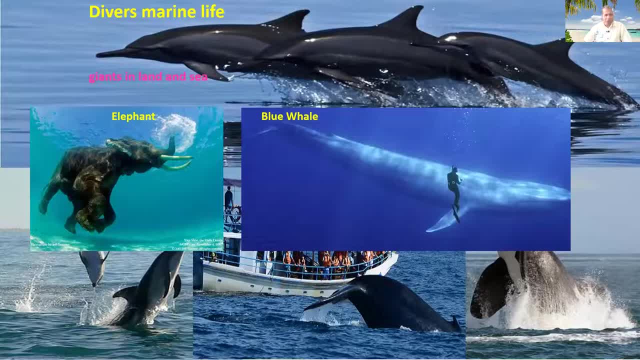 and the aquatic one. they both in our waters and of course, elephant is not in our water, but sometimes, as you can see, they can be in the water as well. but at least within couple of hours time you can see this- both the ocean giant as well as the terrestrial giant. I think nowhere in the world you can see this one. 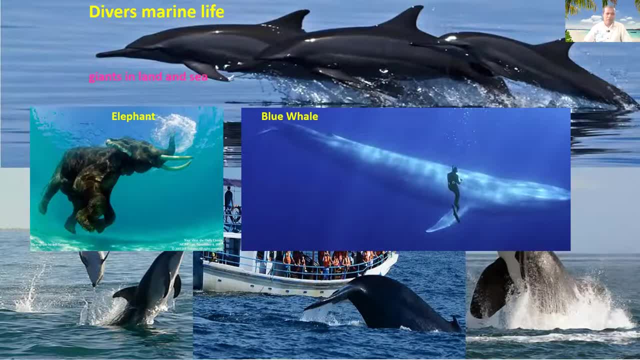 and that's why Sri Lanka has been one of the hotspot for both the terrestrial giant, the elephant, as well as the the aquatic or the ocean giant, the blue whale, or the largest planet that ever we had on our planet, right. so it is something very unique with our country. 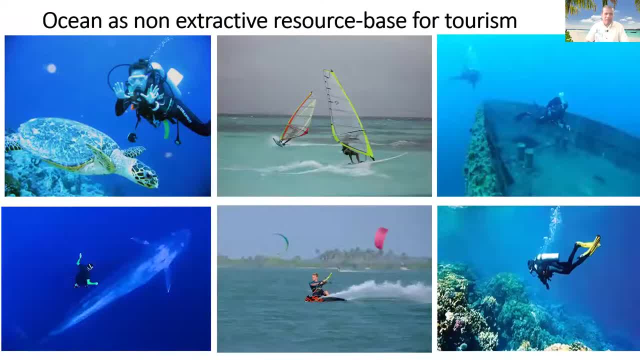 right and, other than that, the opportunities that we have to get the for the recreational purposes, how much we can get out of from the ocean, right from diving to aquatic other sports and diving in the shipwrecks or the diving for the marine mammals as well as for the coral reefs. 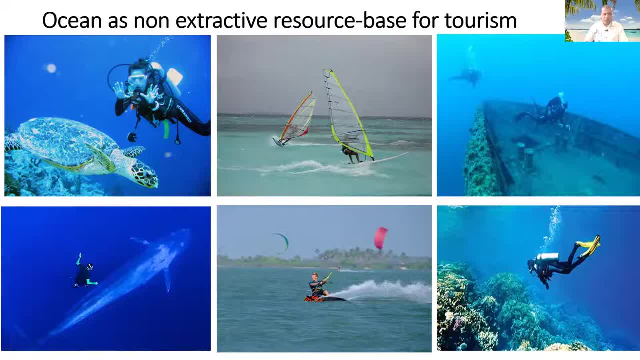 it's a lot of recreational activities and then windsurfing and like kite surfing. now there's very important sport like in the bottom middle called the kite surfing. now the Kalpiti area in Sri Lanka, like, is another world's hotspot for the kite surfing very popular sports among some of the tourists right other than that, this 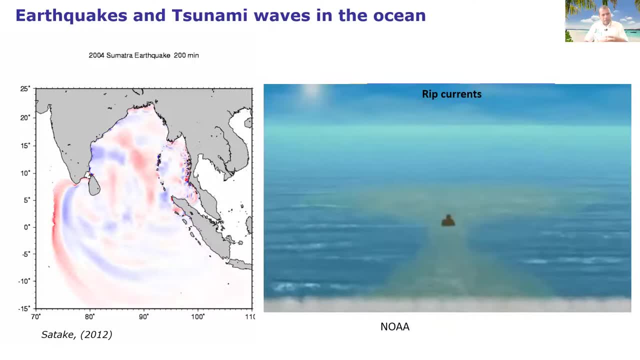 some right the. we talk about the good things, but the bad thing also associated with the ocean, something like this: tsunamis and rip currents, which we will talk about, and I already talked about these things last week as well. we haven't even heard about this tsunami before it happened. at the same time, even the rip currents is one of the. 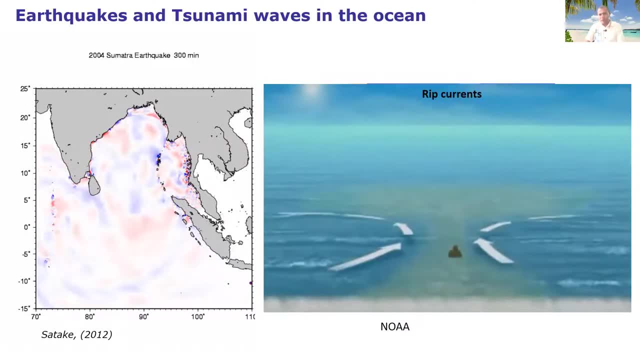 most dangerous the currents that you can see, even in the shallow waters. but very people know about that one because we don't learn about this one and there is no any educational programs to learn or teach people about the rip current, what is it and how to avoid and. 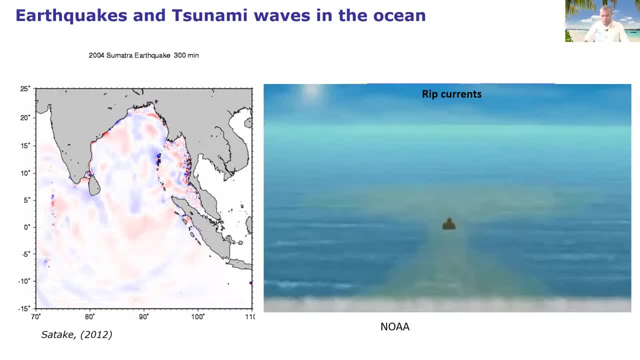 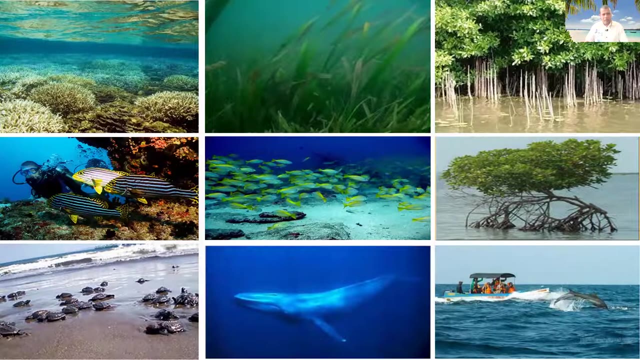 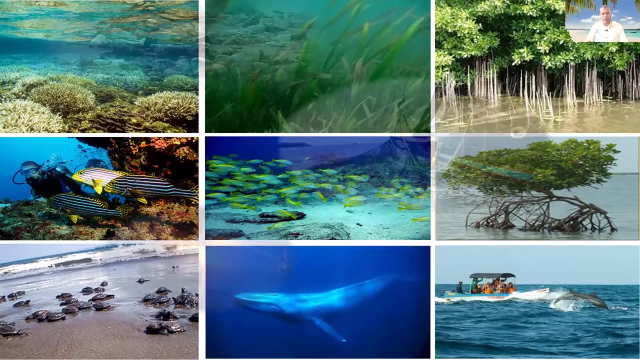 right, that's why, unfortunately, a lot of people get killed by the rip currents. right, we'll talk about these things later on, and from that we see this ocean, all these different ecosystems. it's so much. diversity is all life, this ecosystem. but, as I discussed last week also, 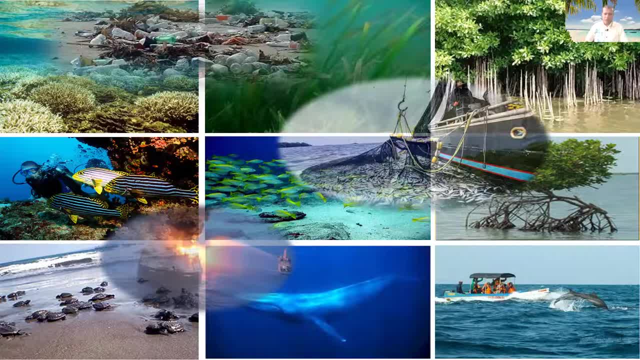 we do, we don't do anything good for the ocean, right? whatever we do, they're all bad for the ocean, right? you can, you can't name and even a single. then we do good for the ocean, right, like like with the, even with this ship accident, right. 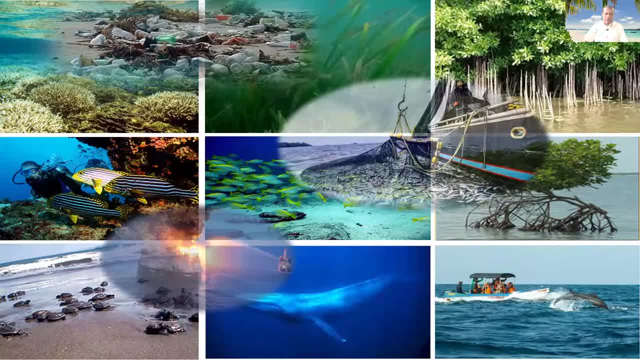 there are a lot of argument about this, but it is not the. the argument is about the, how much the damage it cause or how much money you are going to get, but the nothing in that, the containers or the in that ship going to do anything good for the ocean. that is important, right. 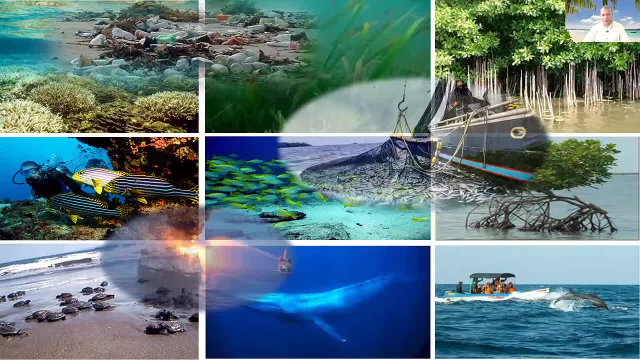 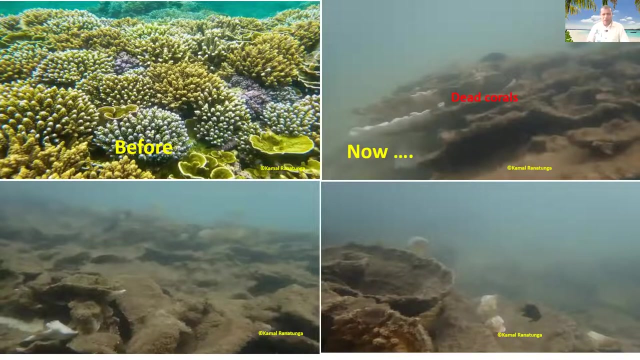 I don't know, maybe even a kissy making, I think, a lot to be in one's in a the layer. is there a lot of, I don't know, because all the water is rain water and in all the whale would be really bad own um and um. we have very sad story about the, the coral reefs. it's not only about the sri lanka, but 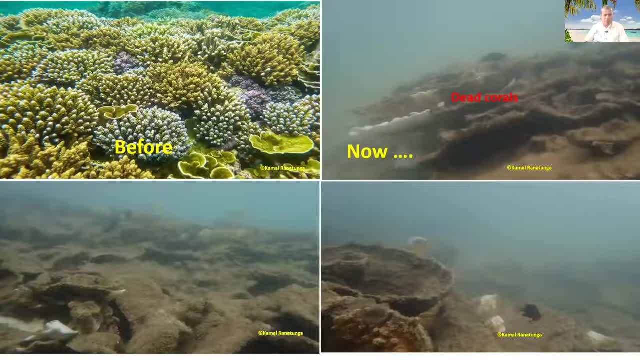 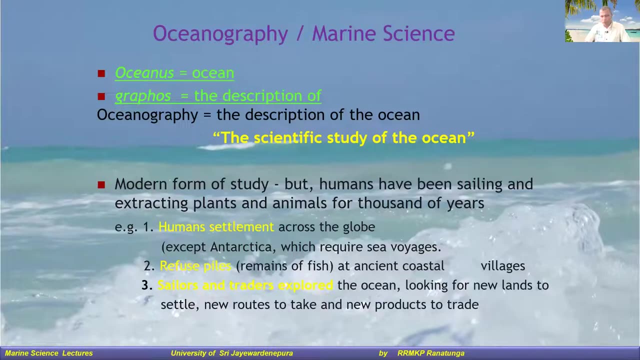 all over the world, even the the largest coral reef, and well-managed coral reef, like the great barrier reef, it's dying. um, so we our oceans as well. right, so that's why we are going to learn about the ocean right, uh, the term ocean, right the oceanography is actually. 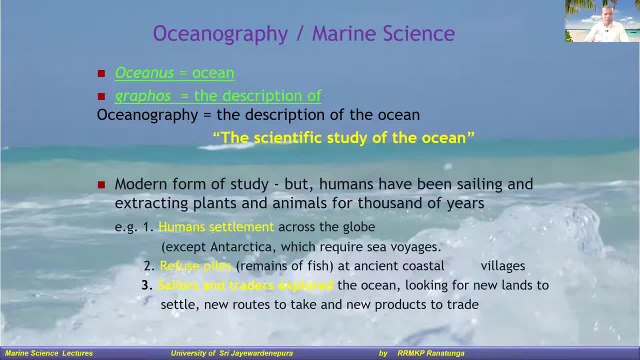 come from a latin terms: the oceanus is the ocean and the graphos is a description. it's more scientifically, we call the scientific study of the ocean. right, you, the? the most important thing with this, uh the subject is that the it's quite recent subject. i am not very recent, but it uh compared to other biological subjects or the physical. 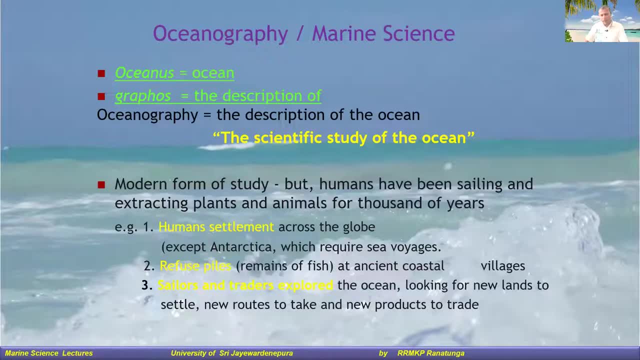 subject like a physics, but this is quite new. uh, but it doesn't mean that the we have not been using the ocean, that we have been using the ocean for so many years. right, we know that the the humans. we know that the the human evolved in the africa, but they had to go to different. 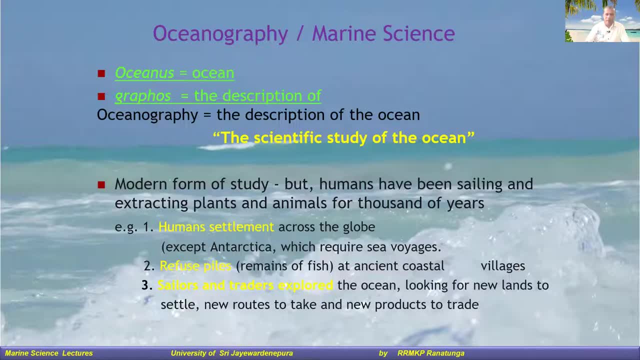 continents and they should have gone to the ocean for the community in the prehistoric time, even right. so definitely there should have been some ocean voyages by even the prehistoric time. and there are a lot of uh we call the refuse files or the any remains from the marine. 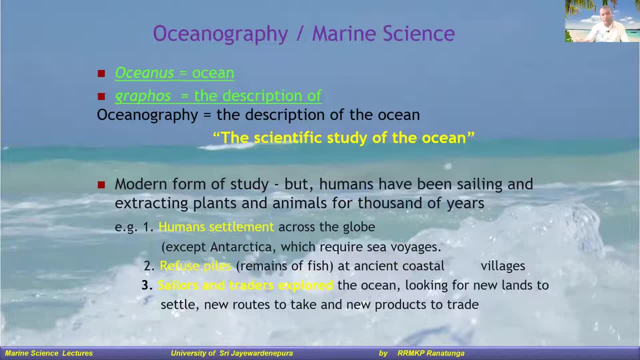 organisms, particular on the fish in the, the ancient or the prehistorical uh habitats or the villages, which means that people have been using fish as a food of some sort of a purpose, right. and then especially the sailors or the explorers, the ocean: they have been using the ocean for quite long period of time, right. so the subject is not anything. new, but i mean not. the subject is: the ocean is a topic of discussion because there are various theories of the ocean, but it is just in the context of that. we have to go back and look at food, for example. so, uh, more and more. but there is a real idea about the ocean in. 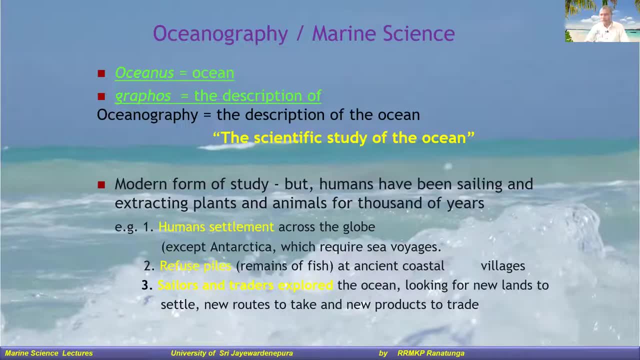 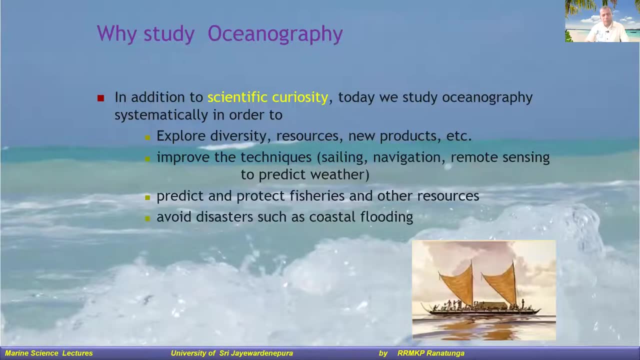 that, in terms of the ocean, it has been introduced from the environment. so, uh, first of all, the is new, but we have been using the ocean for many years now. and then there are a lot of historical background, right in particular the, the curiosity that we had done scientific. 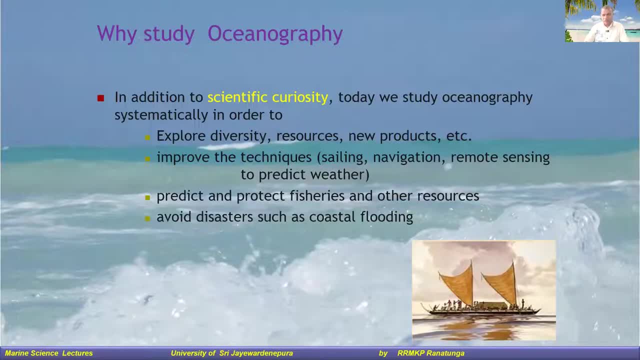 curiosity about the ocean. right, because it's the vast or gigantic environment, and then we know a little about the ocean and then there's a lot of curious things about the ocean. that's why people want to explore. but other than that, there are so many other important 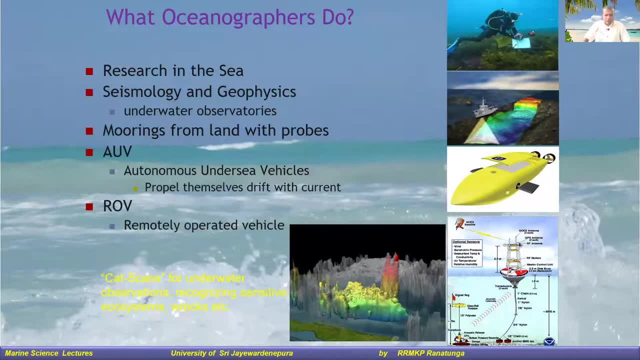 things that we want to learn about the ocean right now. one would think that what are we going to do with the oceanography? I mean doing oceanography right, but if you're really a oceanographer, there are so many things you can be doing. but here you're going to learn. 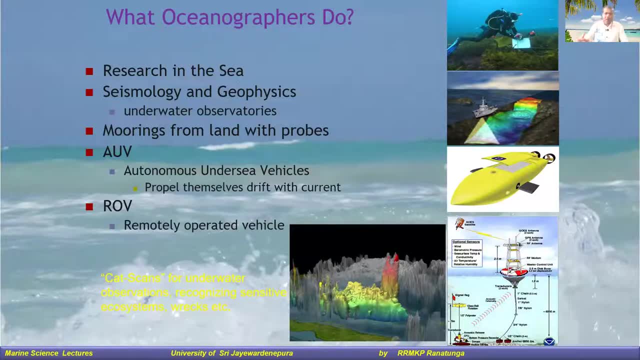 oceanography as a subject, but any of you are going to be interested in oceanography and you will be doing a lot of other things, so I think this is the best way to do it. One thing that we are doing oceanography you can be interested in is how we are going to 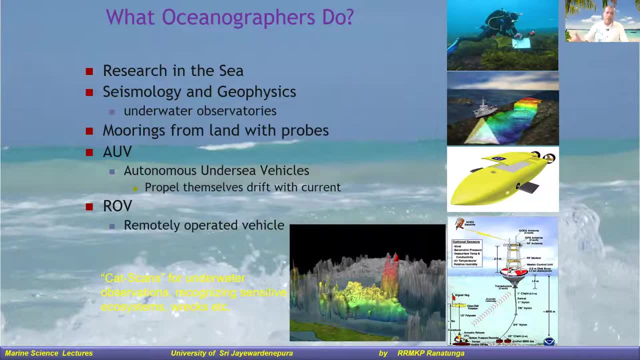 are continuing in this field. there are a lot of things you can do right. especially you can be a researcher in first instance there we- though we are island nation- there are very few people or very few oceanographers. we have, especially on the physical oceanography, chemical oceanographers. we. 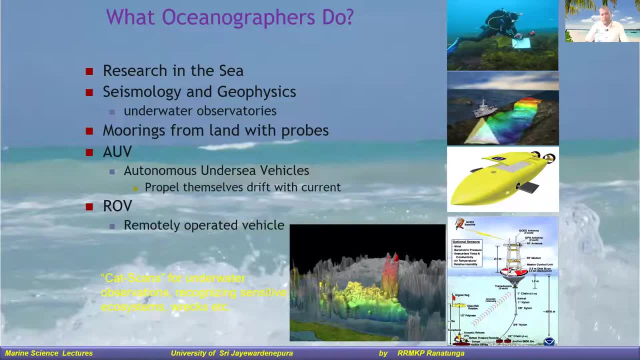 don't really have very few, right? just one or two people in the physical and chemical oceanography, but there are few biological oceanographers. but that's all only couple of people, right. you see, you can't even imagine a country surrounded by the vast ocean, but very few people, very few. 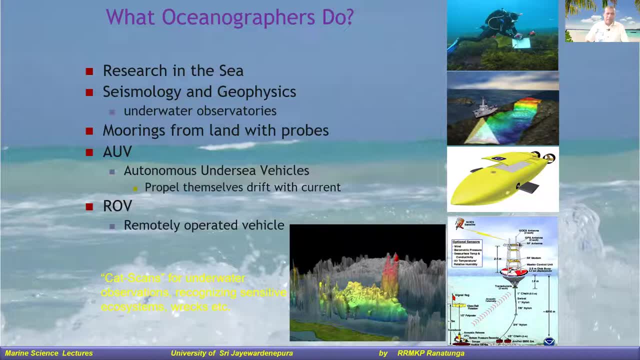 scientists to work on this field. right, and we need a lot of people to work on this, like a seismology, the geophysics, like how the ocean bottom look like, because you no one can see it. so we have to do technology to get some idea about the buttons right. 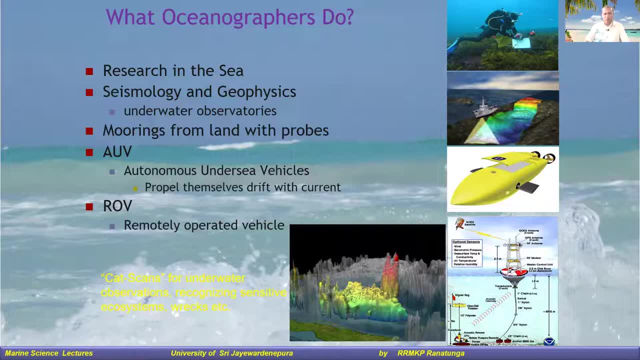 and need a lot of advanced technology, like a uv for the automated automatic autonomous underwater vehicles- right, but we don't have any right. but uh, even some research entities in development they have this kind of thing, but unfortunately we don't have um and remotely operated vehicles, rovs. 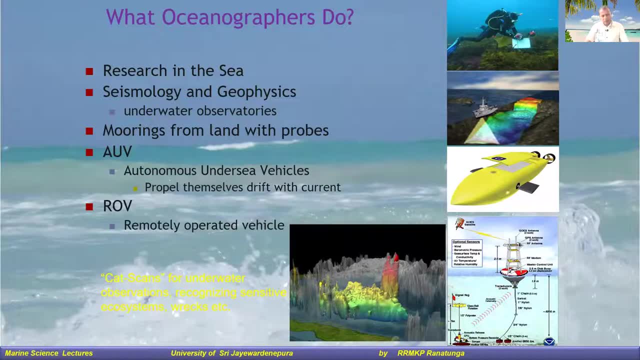 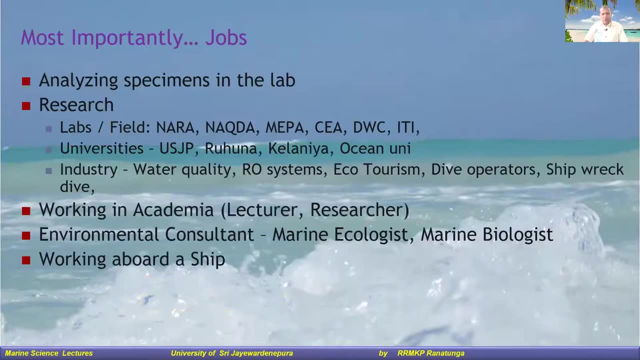 or au is autonomous and remotely. oh, there's two different things like these kind of things. i mean, of course, these are like just to know, uh, some areas you can work, but other than that, um, as i said, you can be a researcher. there are a lot of research institute like like an ara, nectar nepa. 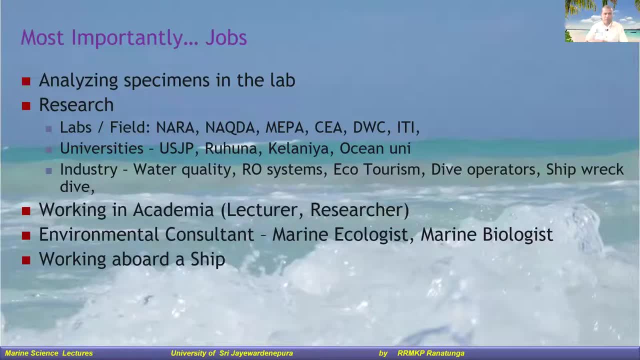 department of wildlife, like research institute, where you'll be working on the ocean related subjects, and also the uh. there is a cross conservation department, of course, different areas where you can work on right and and also you can work in the academia, just like me, right, you can be a lecturer at the same time you can be a researcher, right and environmental consultant. 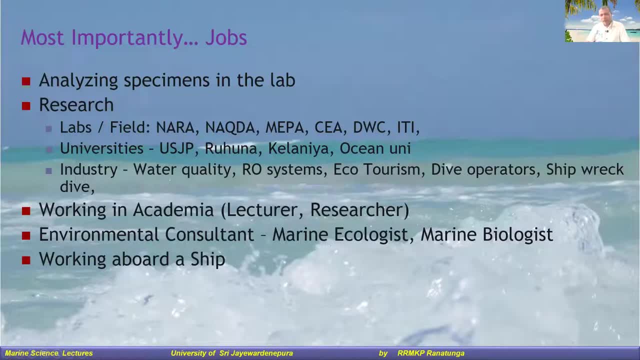 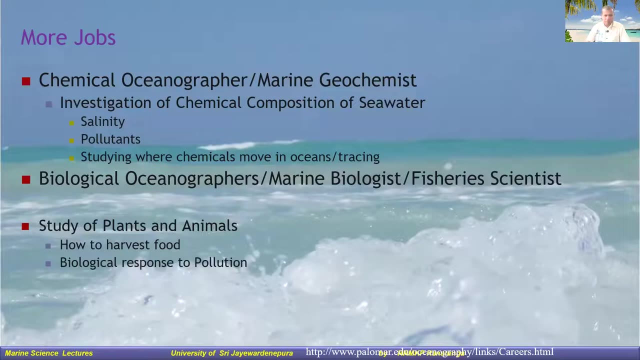 right. there are very few marine ecologists and marine biologists to work in this environment in the field of marine consulting, right, um. so there's a lot of opportunities for people to work right. so i have given even this. i will share all this with you later on. 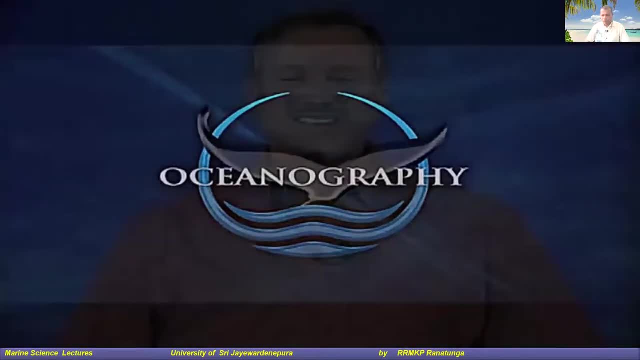 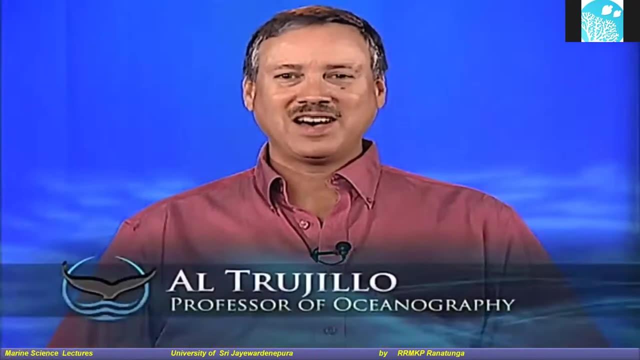 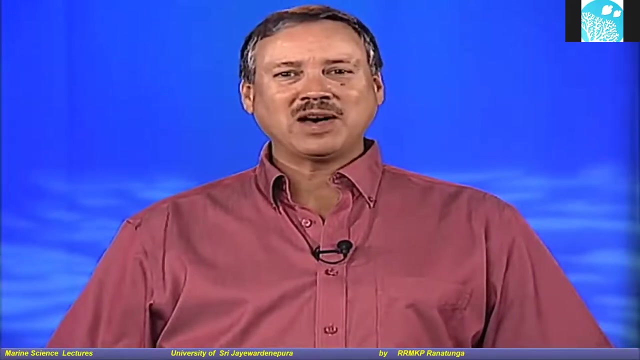 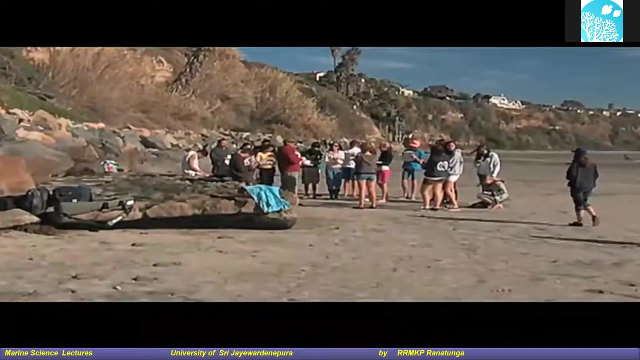 you want to know more about oceanography. why oceanography if you're interested in the ocean? right now, we're Die придум. hello students and welcome to oceanography 100.. i'm al terhill, professor of oceanography here at palomar college and lead author of your textbook. i want to tell you a little bit about this course. 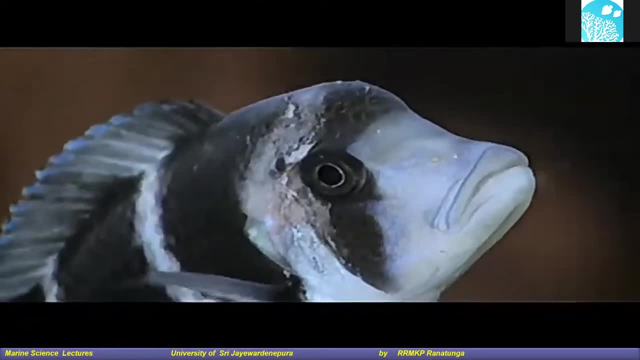 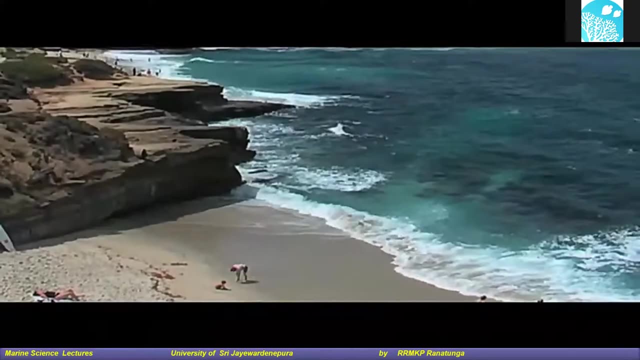 hope that it elicits a sense of wonder and a spirit of curiosity about our watery planet. The ocean represents many different things to different people. To some it is a wilderness of beauty and tranquility, a refuge from hectic civilized lives. Others see it as a vast recreational 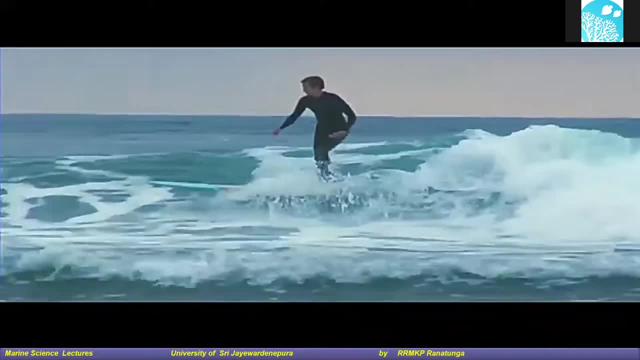 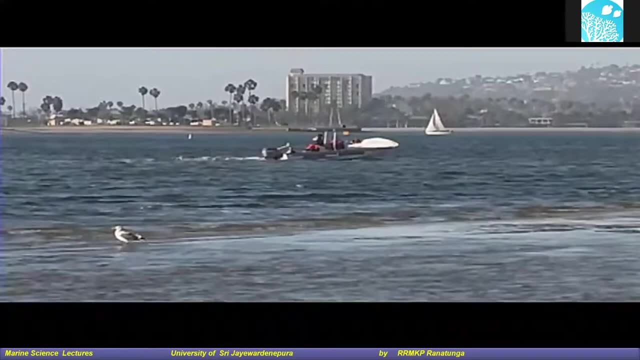 area that inspires either rest or physical challenge. To others, it is a mysterious place that is full of unknown wonders, And to others, it is a place of employment unmatched by any on land. To be sure, its splendor has inspired artists, writers and poets for centuries. 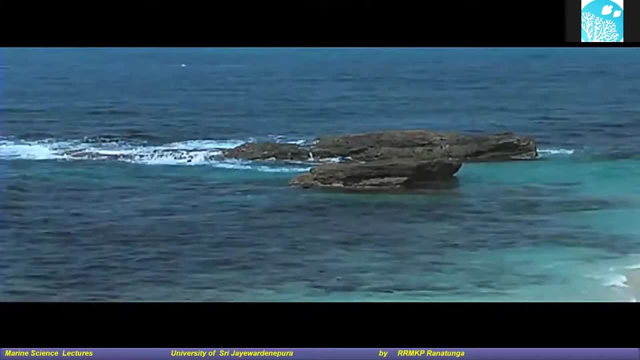 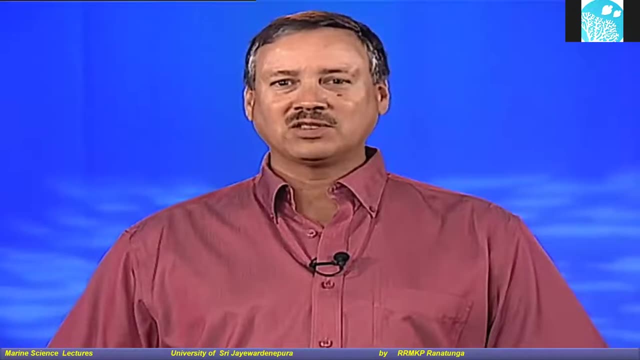 Above all, take time to admire the oceans. The scientific study of oceanography is typically divided into four main academic disciplines or sub-fields of study with much overlap. They are first: geological oceanography, which is a study of the structure of the 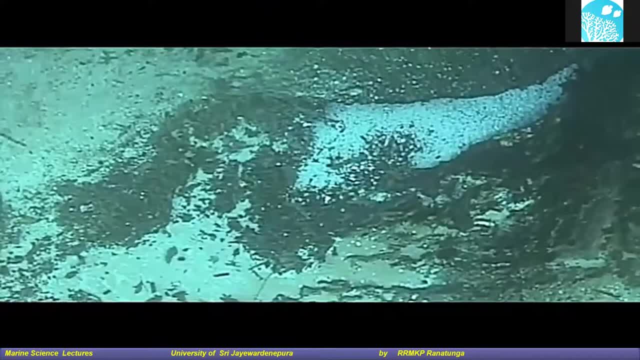 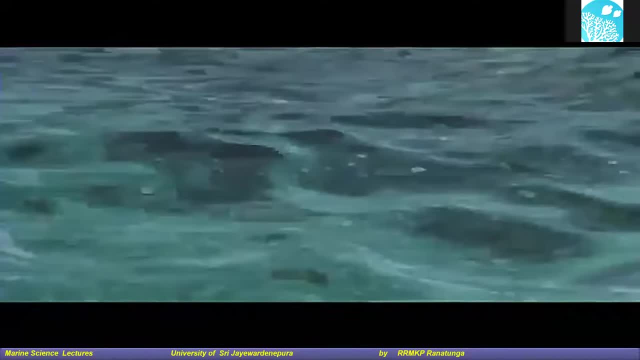 seafloor and how the seafloor has changed through time, the creation of seafloor features and the history of sediments deposited on it. Second, chemical oceanography, which is a study of the chemical composition and properties of seawater. how to extract certain chemicals from seawater. 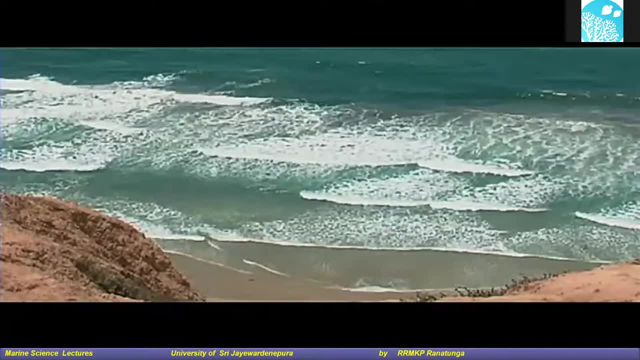 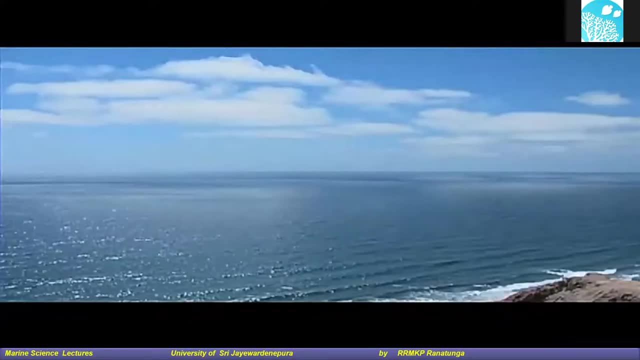 and the effects of pollutants. Third, physical oceanography, which is a study of waves, tides and currents, the ocean-atmosphere relationship that influences weather and climate, and the transmission of light and sound in the oceans. Fourth, biological oceanography. 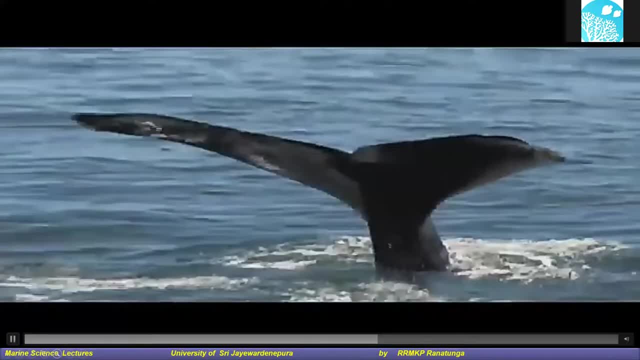 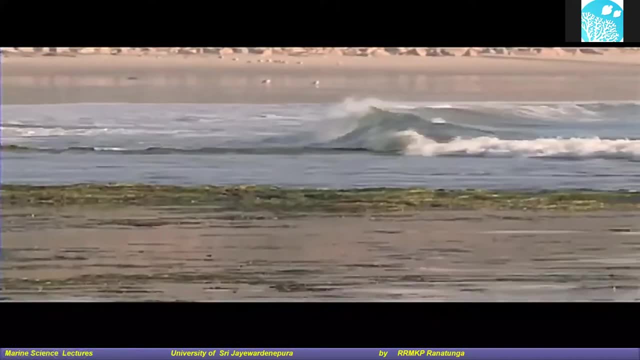 which is a study of the various oceanic life forms and their relationships to one another. In this series of information, we will also take a look at a few of oceanography's most common lateral main functions, such as natural environment adaptation to the marine environment. 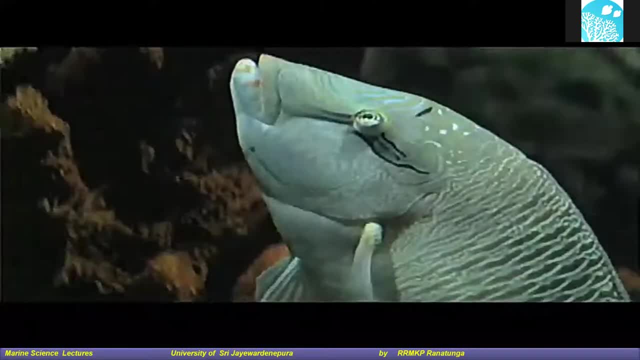 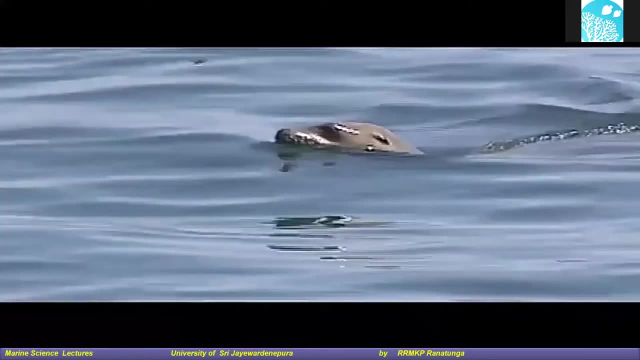 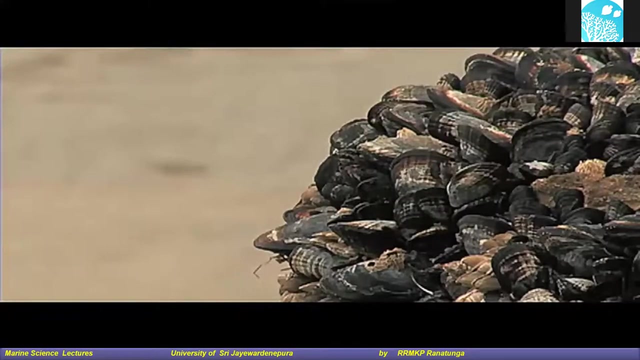 and developing sustainable methods of harvesting seafood. Other disciplines include ocean engineering, marine archaeology, ocean policy and marine education. Because the study of oceanography often examines in detail all the different disciplines of oceanography, it is frequently described as being an interdisciplinary. 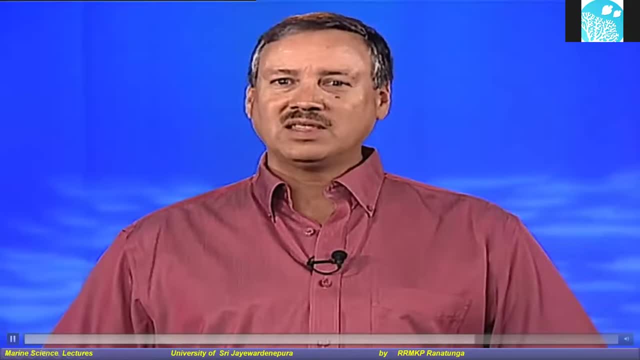 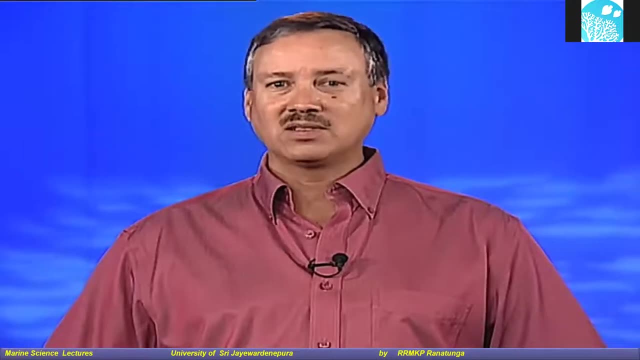 science, or one covering all the disciplines of science as they apply to the oceans. range of interdisciplinary science topics that comprises the field of oceanography. In essence, this is a course about all aspects of the oceans. Lastly, the content of this course was carefully developed to provide a foundation in science. 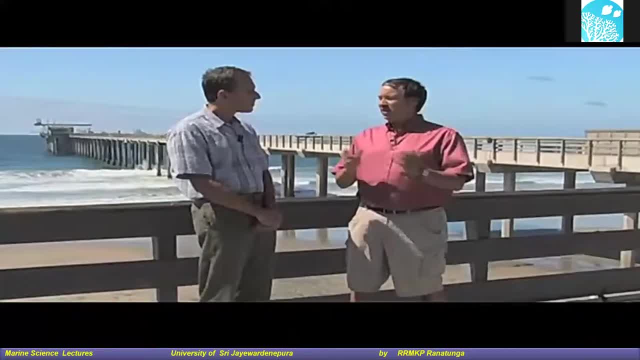 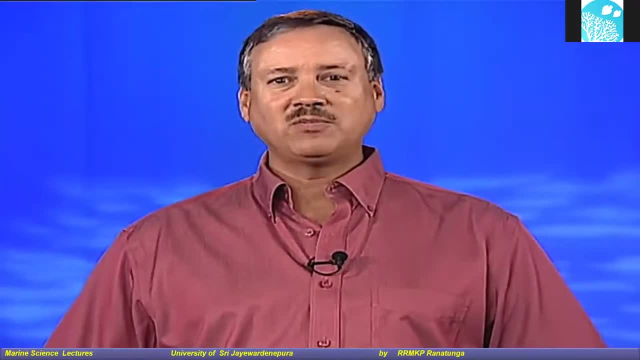 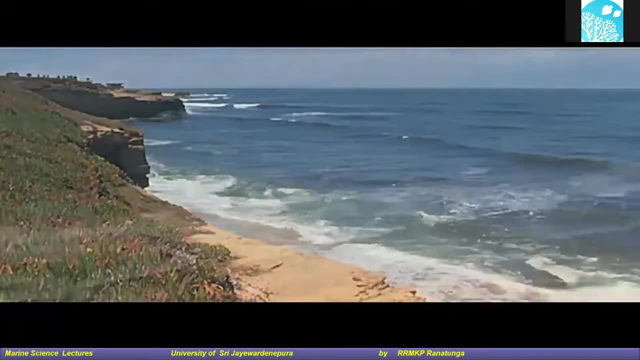 by examining the vast body of oceanic knowledge in an educational and sometimes entertaining way. My desire is that you will take away from this course much more than just a collection of facts. Instead, I'd like you to develop a fundamental understanding of how the oceans work really. 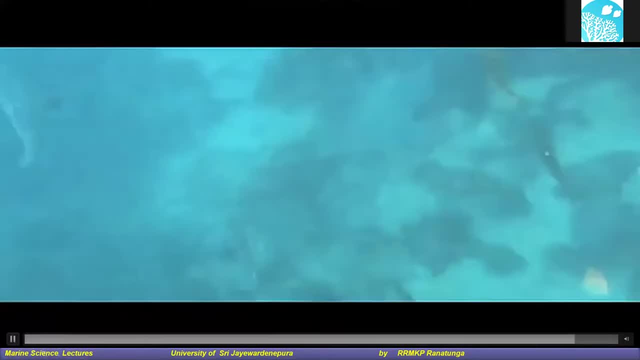 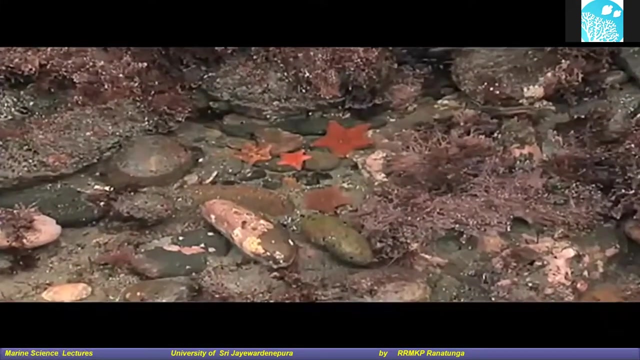 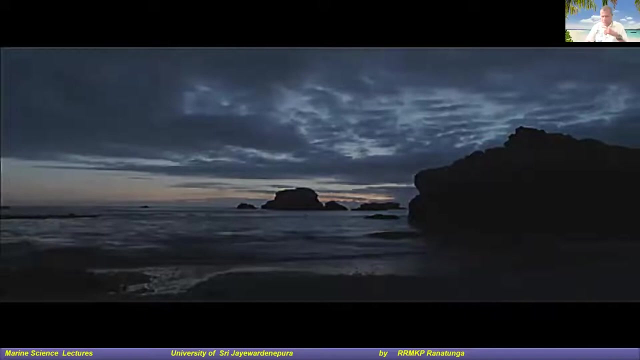 why the oceans behave the way they do. In the end, I hope that understanding the way the oceans work will foster an appreciation of the marine environment and a desire to help preserve it. I hope you enjoy this course. Hi, I just showed that video because he is one of the authors in the one of the textbook. 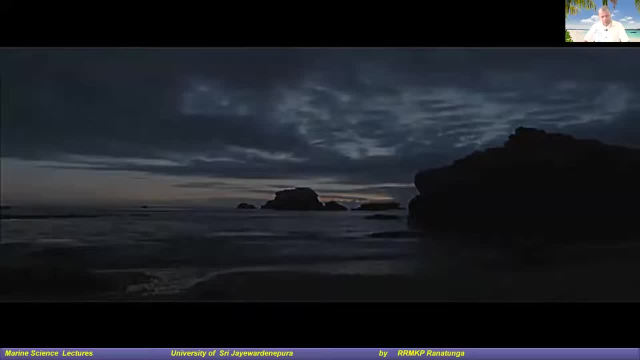 in the oceanography as well as a researcher in the oceanography who is also a teacher. I just want to show you that, what you are going to learn in this course. Thank you, Thank you. So I'm using the election series as a light. 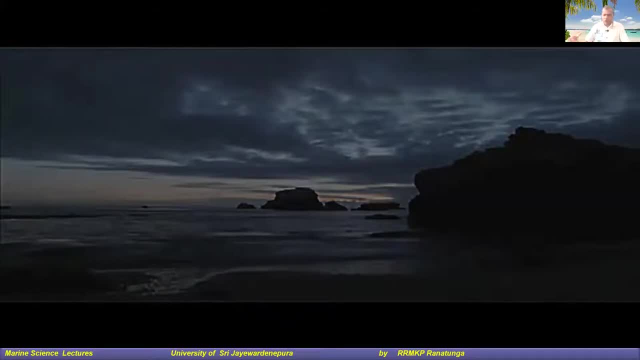 So never underestimate that we have gone to what the the world sells right, staging how that teaching, what is teaching in the best universities in the world, And we are getting some insight or getting some ideas from home from them how they are teaching and also adapting the same thing or not. 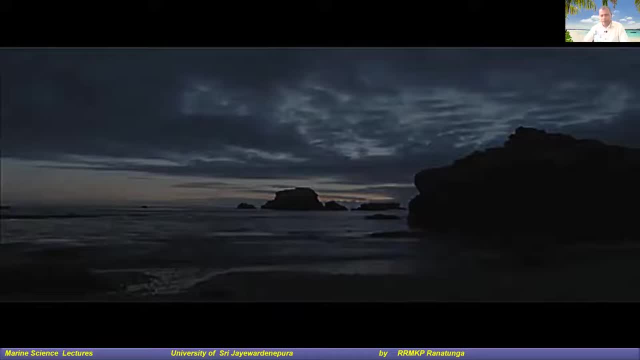 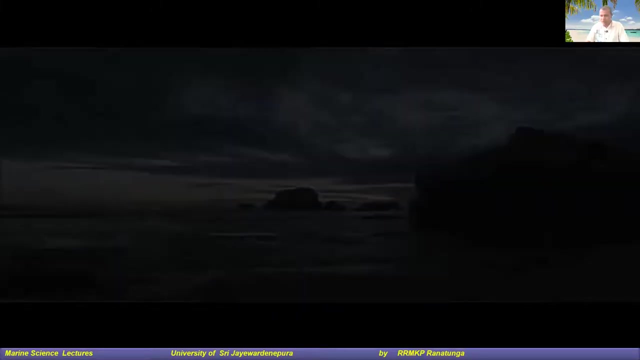 The same thing, but with be the best thing that we can use in for us, them in for our purposes as well. that's why i'm so. so i hope you can get a- i mean sort of a maximum out of this course on the particular subject, right? um, just to give another few things, uh.